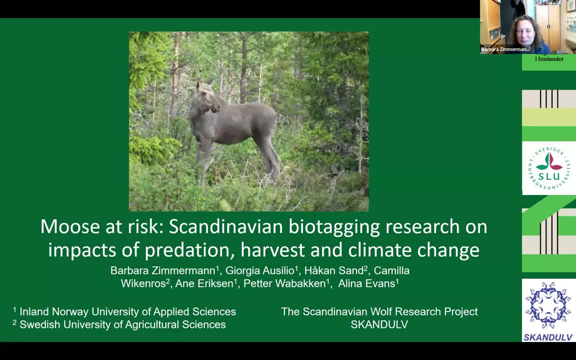 and other research And it was nice to host her at our place And she was contributing a lot also with her field work And she was helping us with the Wolves to Cross Borders conference And we had in May. So I'm originally from Switzerland but I've been living more than 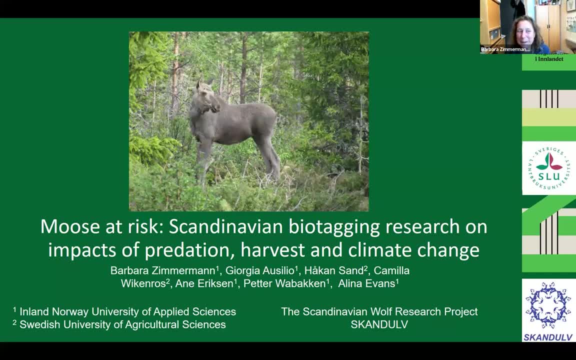 half of my life in Norway And I have done my PhD here in Norway, And I also I'm working here Now still, and I'm both teaching and I'm also doing quite some research, And so so the study that or that, what I'm going to present to you today, is about our research. 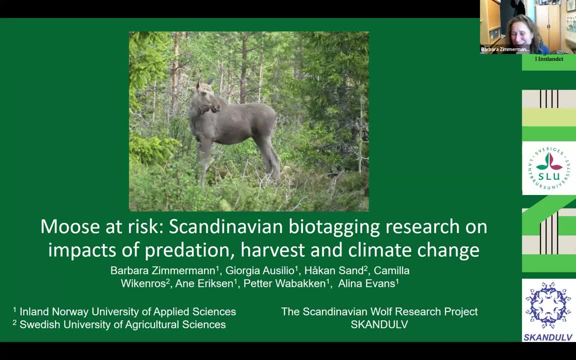 on moose. I've just heard that you've had the first moose in Hungary, So this, so then you can get a bit better prepared on what you can wait for. It's actually very interesting because moose is a species that is very well adapted to cold environments. And look at. 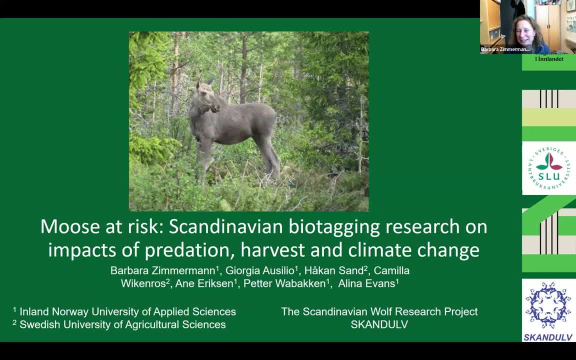 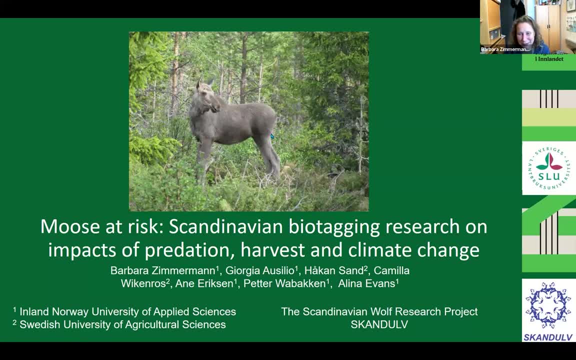 and it has very, very long legs. So, and why does it have so long legs? because it's optimally adapted to a lot of snow And so we can walk through the forest and he's not hindered by one, by by a half meter of snow, or. but then, when it gets higher than 70 centimeters, then 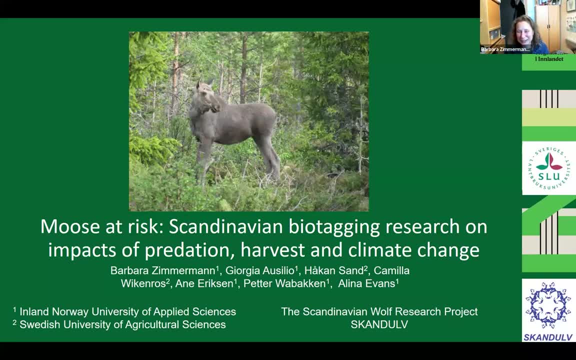 then it's a moose get kind of, can get a bit more stuck or they get. you know they're don't move that much anymore, but so they are really well adapted to snow and to cold environments. also in our latitudes the moose have like their optimal winter temperature at minus 10 degrees. 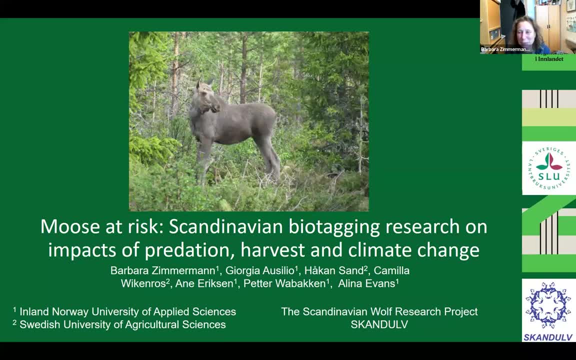 um, and in the summer it's just above like zero, maybe plus 10 degrees, but but so they're. they're really, uh, well adapted to this um, cold environments and boreal forest, and so i think it's also really exciting now to see this expansion of the moose um into their earlier habitats. uh, so they definitely. 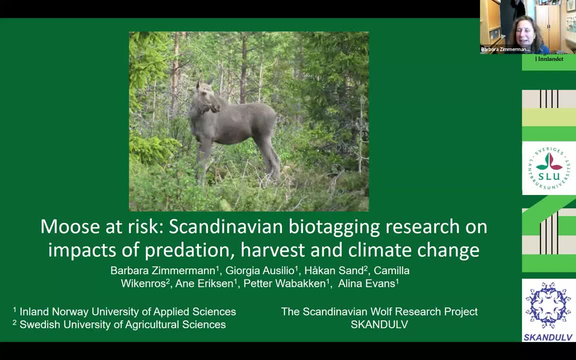 also can make it in temperate environments, um, and they have been in those places in central and western europe before, uh, in more temperate forests, so it seems like they are kind of adaptable. it's an adaptive species, so it'll be interesting to to learn more about the moose also in the 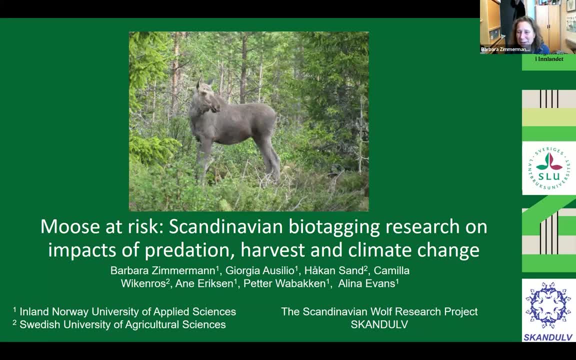 southern region, but for now we keep to scandinavia and to the, to the boreal forest. as you see, there are many co-authors that, so i'm not alone on this. i have very good colleagues working together with on on moose, and they are both from my university but also from the swedish. 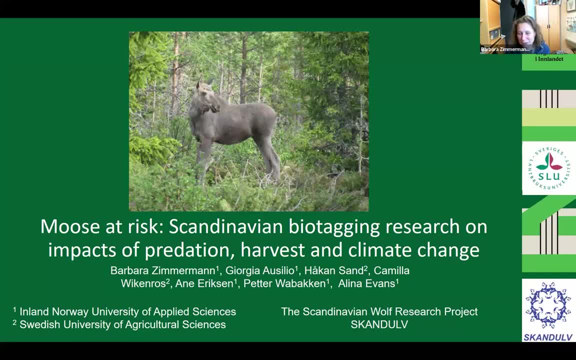 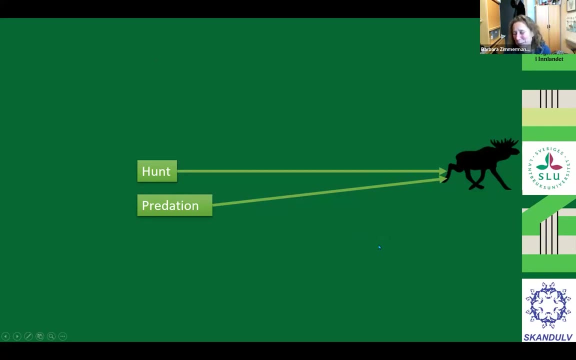 university of agricultural sciences from the grimsey research station. um, let me see it doesn't work yet. now it works. yeah. so the moose, um uh, is exposed to many risks. so the title was moose under pressure, and what are the pressures on moose? yeah, the first thing, uh, we think of is uh, 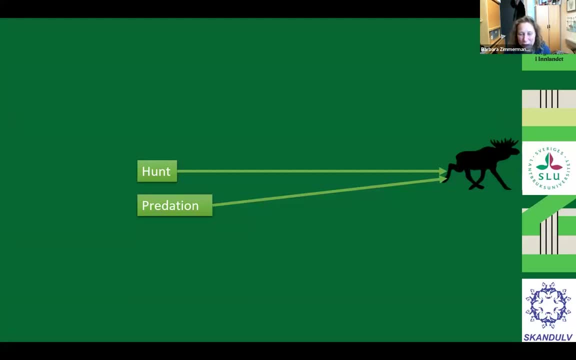 is predation and hunt uh or harvest, that's kind of a direct mortality um, and definitely uh is a kind of the main factor regulating the moose populations in here in the boreal forest um. but then we also have more indirect effects on moose. we have uh infrastructure development uh, for example. 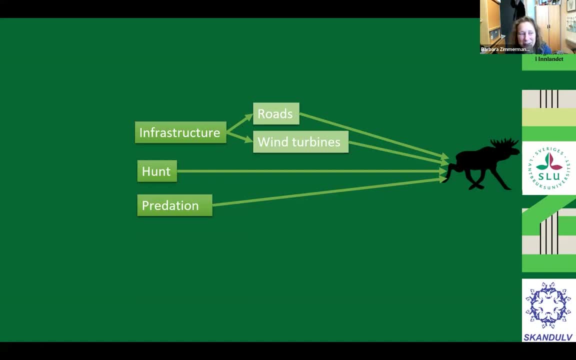 the building of roads. uh, we have a huge network of forest roads in the boreal forest to exploit the forest resources and this network is expanded and the roads are getting broader because they bring their big forestry machines into the area. also, we see a lot of wind power development in 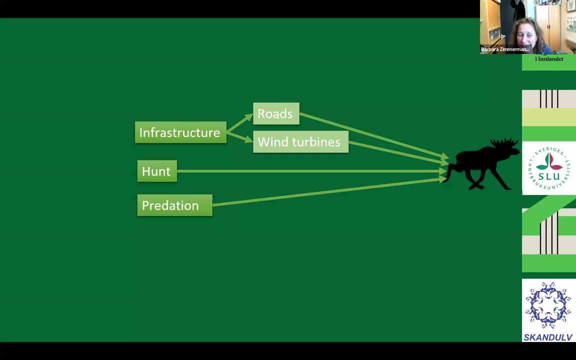 scandinavia, also in the forested areas, not only along the coast and on the mountains, but also in forests, and so this has also might have effects. we don't know yet, but it might also have effects on moose. um for sure, forestry is a very important factor. 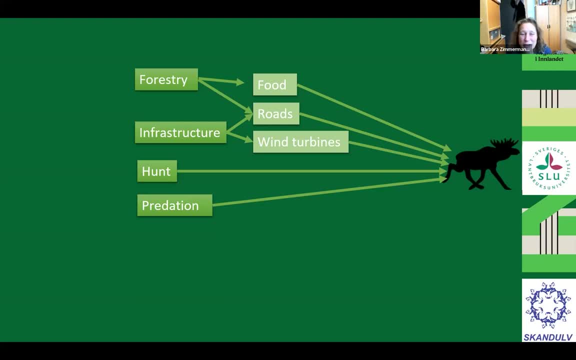 um, i already talked about the forest roads, but actually forestry can also be positive because, um, in the 1950s we have started to use clear cutting as the main forest management or as the main way how to to extract the resources out of the forest. and with those clear cuts, uh, we get. 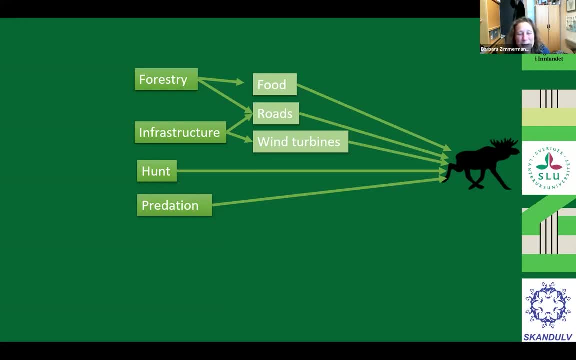 these hot spots of uh, summer food. uh, because, for example, we have, uh, we have, uh, we have a lot of. we get a lot of new fresh vegetation coming up and raspberries and fireweed and like different perennial plants, but then also a lot of deciduous tree species that come up, because there suddenly 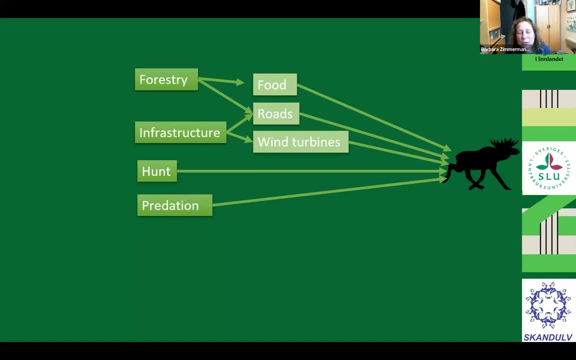 there is a lot of light, um and so for like for a while, for like maybe 10, 12 years. these uh clear cuts into into very resource rich areas and this was one of the main reasons why the moose population in the after the like in the 1970s started to explode in scandinavia. so we had an incredible 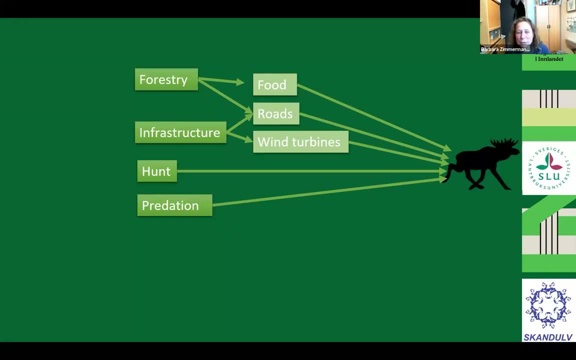 increase in in a number of moose um. but the other reason also is that we had got better hands on the harvest. so we started to have a quota based harvest system, um, where different sex and age categories were targeted um in in a way, so that we could kind of optimize the harvest. 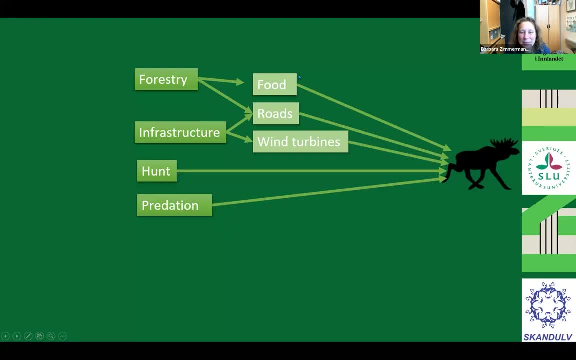 but yes, forestry important. it comes with a lot of food, but on the other side it can also have negative effects through forest roads, and then we have the weather is affecting the food resources. in dry years we will not have that much productivity, um, and and moose actually can starve. one of our most important weather variables is the snow. so, um, the snow here. 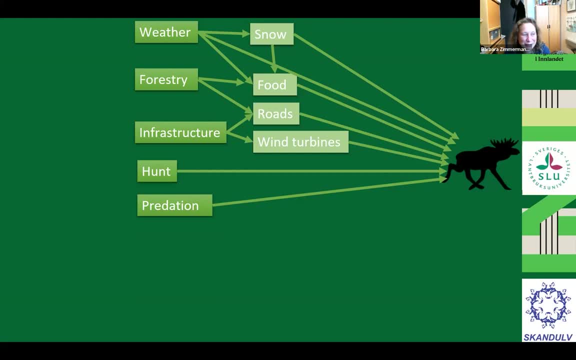 in even stuff where i work now. if i could, maybe i can show you on my camera. if you can see my camera, it's white and nice and snowy right here out there now. So the snow is. we have snow layer from like mid November to end of April, So half of the year for a moose is. 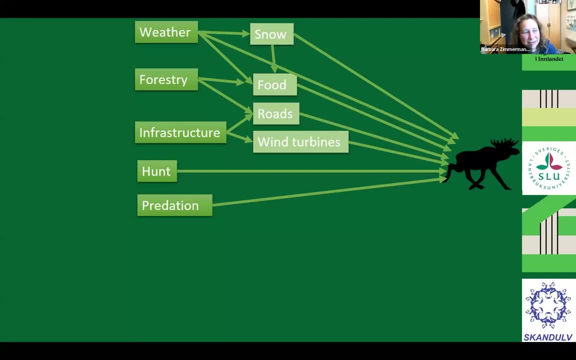 kind of covered in white And the snow doesn't only cover kind of our trees and whatever, but it also covers the food of the moose. Moose don't anymore than have access to the, to the field vegetation, So and also snow can if it's too much snow, if it's 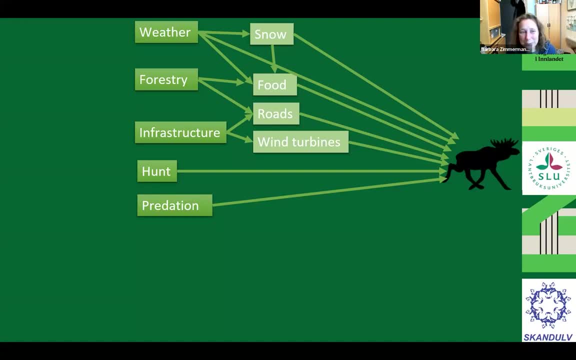 more than 70 centimeters, it will also hinder moose movement. It's a very important variable But, as I also said, dry summers can be detrimental for moose. If it's a coolish kind of rainy spring and summer, that is more positive for the moose because 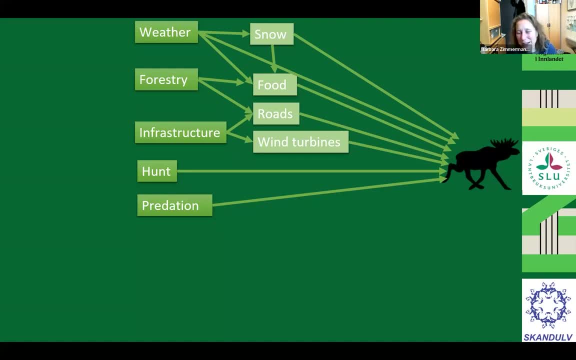 then the plant development is slower and more productive. Then we have a competition. There are other species in the forest that might eat the same things as the moose. I'm thinking a bit about the roe deer, red deer, Red deers are mostly grazers, but they can. 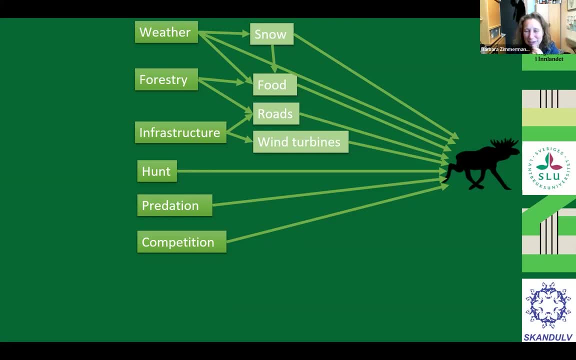 also in, especially in the winter. they also like to browse on on trees And they also in the like in the fall and in the spring. they eat a lot of heather in the forest, for example bilberry and bilberry plant, So there might be some. 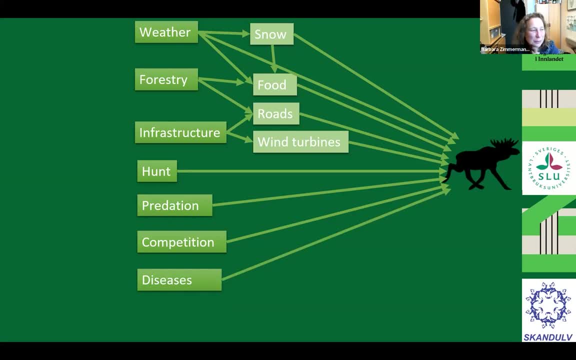 overlap, dietary overlap, but we don't actually know too much about competition between those species And diseases- is another pressure on moose. We have, for example, a new disease coming, or let's say more, it's more a parasite. I won't call it really a disease yet, But 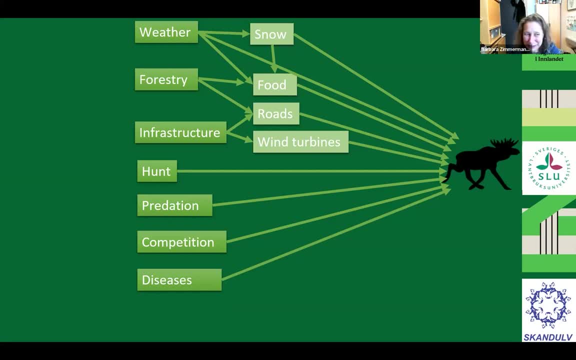 we have a parasite- This that you have a lot. I know you have a lot of them in Hungary. It's the deer fly And that's a new element in our regions and also for the moose, And but there are also other kind of diseases. 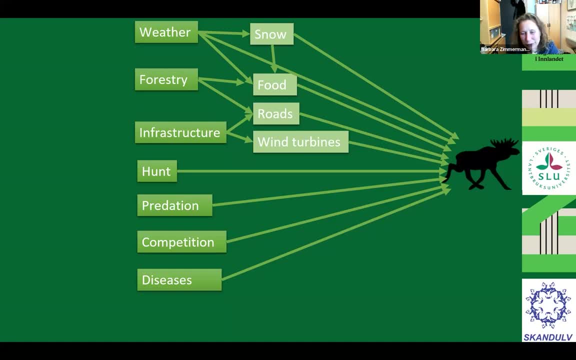 And we have now found some echinococcus, for example in moose, and so hunters are a bit concerned about that, And diseases can be spread easily if moose gather close together, And that happens especially when there is supplementary feeding of moose. And why would there be? 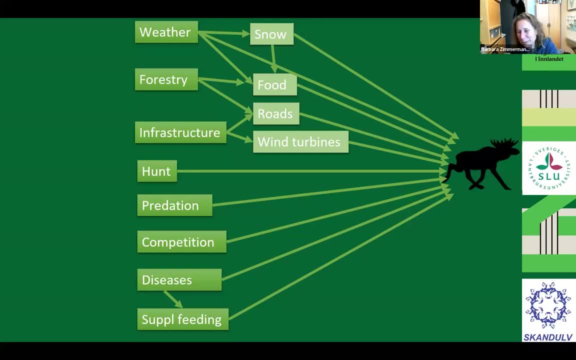 supplementary feeding? Yeah, because there are several reasons why it is done in some areas of Scandinavia. Partly it's to keep the moose away from the roads- And here I don't mean the forest roads that I've been talking about, but I mean the big roads, because we have those collisions. 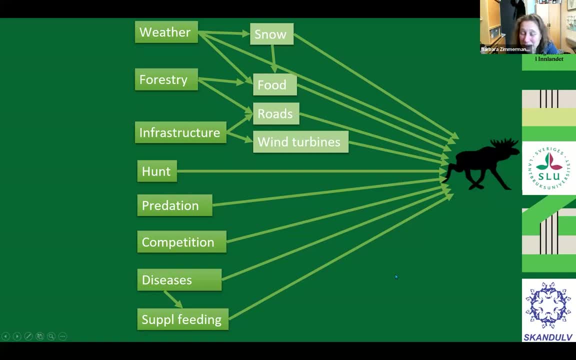 with moose. they can be detrimental not only for the moose, but also for the, for the car or the people involved. Other reasons for supplementary feeding is to keep them away from young forests, So they won't make too much damage to production trees or 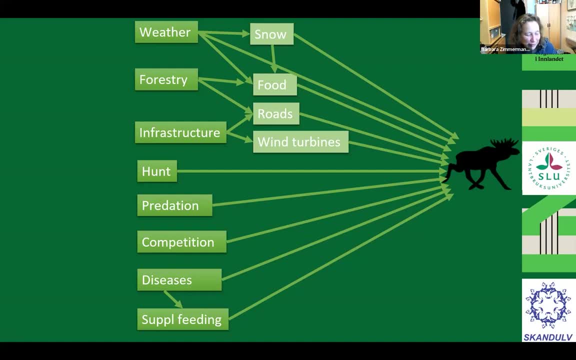 just to increase the productivity in the moose population. So there are several reasons why it is done. But actually it has been in Norway. now it has been forbidden to do supplementary feeding Because we have had a first outbreak of chronic wasting disease in, even though it was in reindeer, in wild reindeer. it is kind of we. 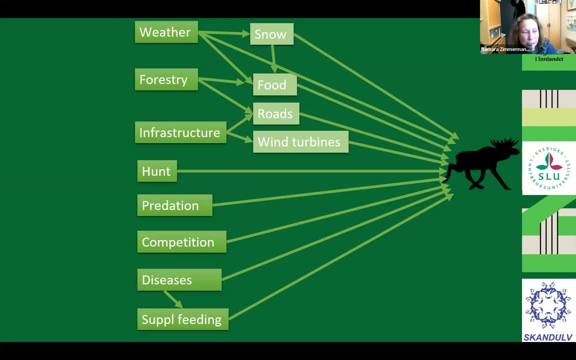 don't really know yet if this disease or this prion disease can go over to moose, So that's why it has been stopped. But the landowners can still apply for it and they can get some exception from the law if they have some good reasons for that. So a lot of. 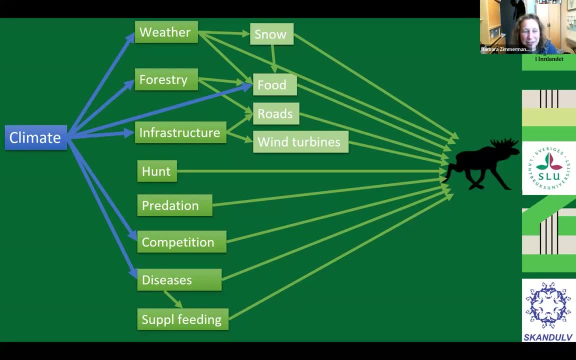 factors here, And many of those factors are actually driven by climate, Like the weather, the forestry infrastructure- when it comes to wind power development, for example, And so on. So the climate is kind of a main factor in the background that influences a lot of those factors that affect moose. So my 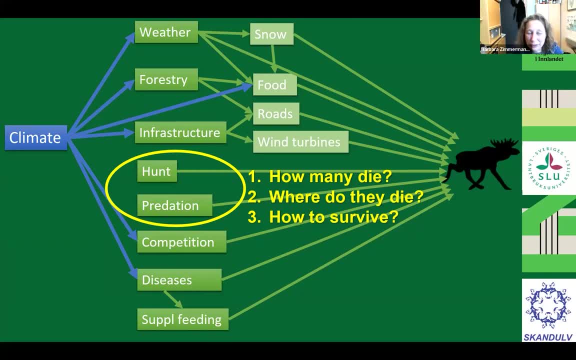 talk today is: I will talk more about harvest and predation, and I will first tell you a bit about how many moose that die, And then where do they actually die And how can they survive- survive in these risky times. And then, in the end, I will talk about upcoming research on climate change impacts. 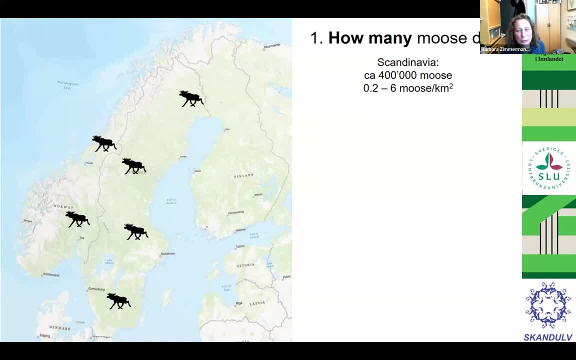 So the first question: how many moose die? So in Scandinavia we have about 400,000 moose, And if I say Scandinavia, I mean Norway and Sweden. Finland is not a part of Scandinavia. Finland is a part of the Nordic countries that we also belong to. 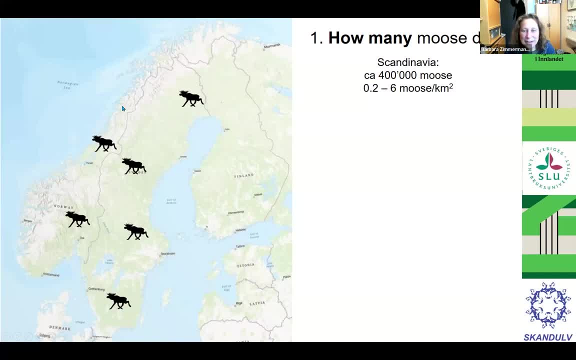 But so if you just look into Norway and Sweden, isolated like this peninsula, here it's about 400,000 moose And the densities differ a lot. We have some areas with very low densities, especially those areas that were in the winter. 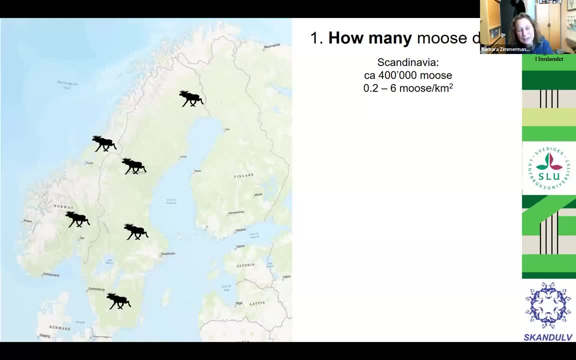 when the moose migrate out of those snow rich areas And then they can have very, very low densities, But then again they can gather and have Kind of high densities in winter concentration areas. Annually one out of three to four moose are shot every year. 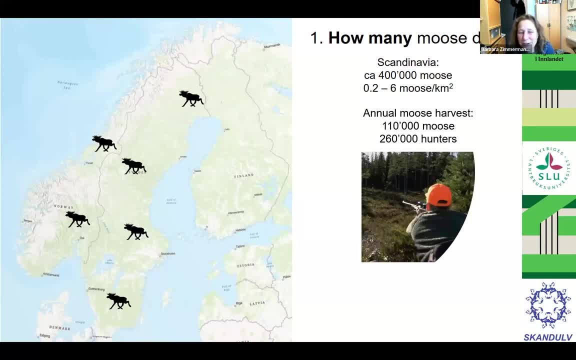 So 110,000 moose are harvested And we have 260,000 hunters registered annually as moose hunters. So 260,000 hunters that buy a license And then we have about 150,000 hunters registered annually as moose hunters. 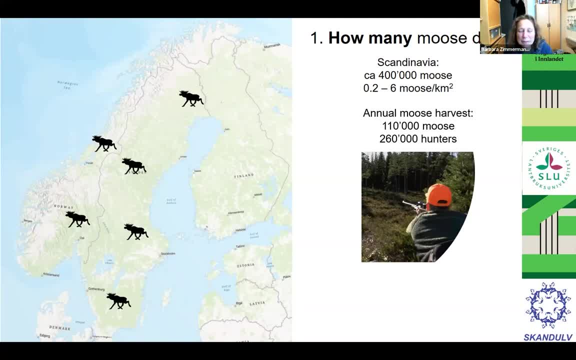 So 250,000 hunters that buy a license. So you can see that it is a very important cultural event. actually, Every fall moose harvest is kind of That's. for many people it's more important than Christmas and Easter together. 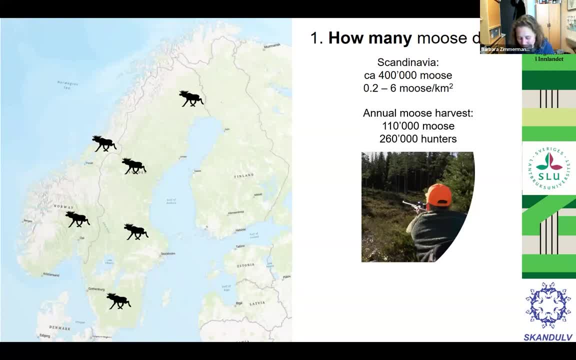 So it's an important time And it is also kind of a strong cultural heritage in these two countries. Okay, And then we had the wolf. that returned into this area. Wolves were extirpated in Scandinavia, But there were wolves surviving in Finland and chasing areas in Russia. 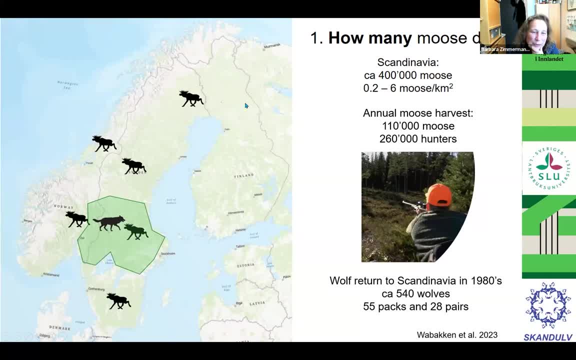 And so wolves immigrated into this area here and established a population, And now the population counts about 540 wolves with about 55 packs and 28 pairs, And most of them are on the Swedish side And a little bit on the Norwegian side here. 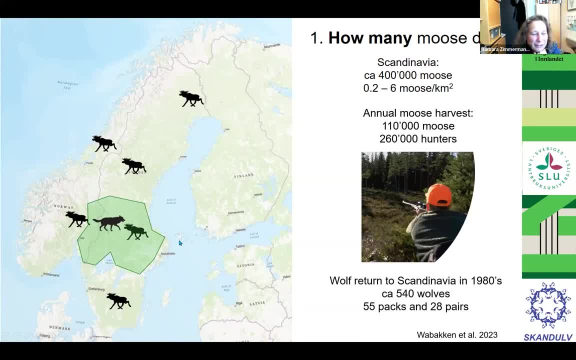 You might maybe wonder why they are kind of concentrated down here And there is no wolves here. This is because here in this area, we have the semi-domesticated reindeer, So we have this reindeer husbandry, which is a traditional background, but also one. 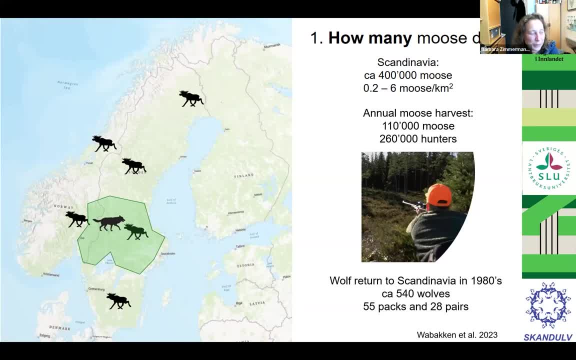 of the most important animals in this place. Some of the animals we have in this area traditional Sami way to produce food in these very production-poor areas. So both Norway and Sweden have decided that the wolves are unwanted in this area here. 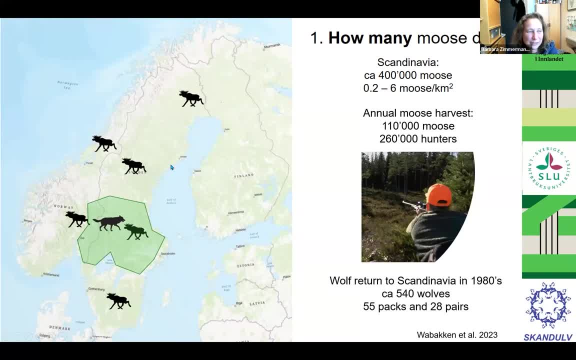 so there is no wolf establishment allowed. As soon as there is a pair that tries to settle, they are either shot or they are moved into this area here. Also, we don't have more wolves in the western part of Norway here, and this is because we 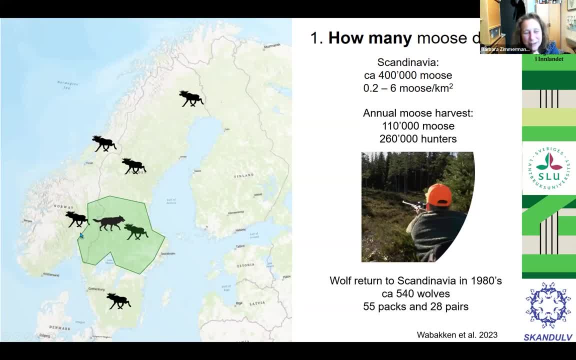 have a lot of free ranging sheep in the summer in these areas and again it is a political decision to not have any wolves allowing to establish in this area In the south here Sweden, and wolves are coming now more and more and I guess in the next two, three years we will. 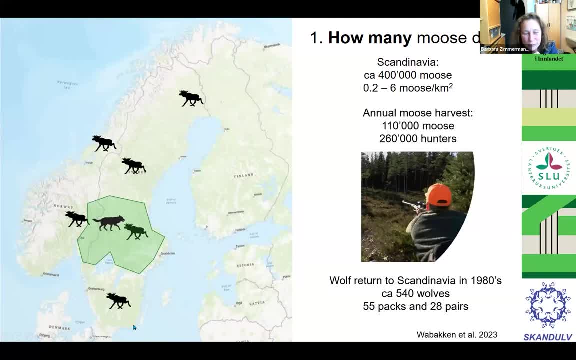 see an explosion of wolves in this area. here there will be a lot of wolves establishing. we have already now three, four packs in this area here down in the south, and I will. there are more to come from this. so it just takes time for them to establish because there is a major motorway. 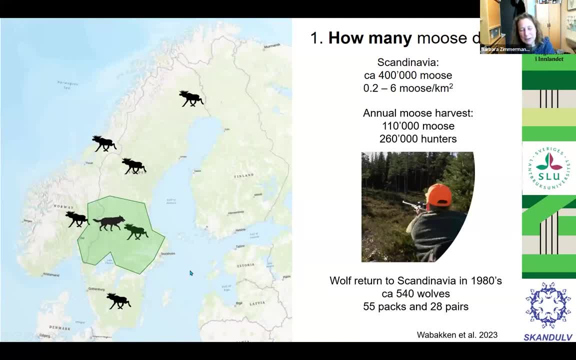 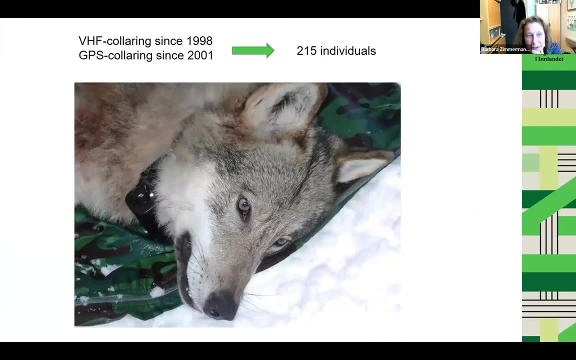 between Oslo and Stockholm. that kind of stops some of the of the spreading of the wolves, but it will now I think that they kind of the process has started so there will be more wolves in the south. We have started our project that is called Skandul, the Scandinavian wolf research project. 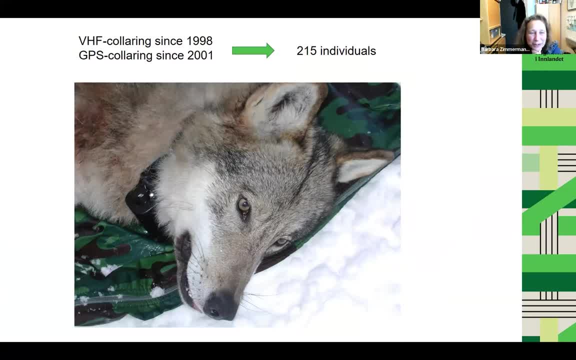 in 1998 with the VHF coloring first, and then in 2001 we started to gps color wolves and so far we have colored more like 215 in different individuals, some of them for several years. so we have a lot of data on wolves and actually the first coloring of wolves we have done- or like the gps coloring was done to actually 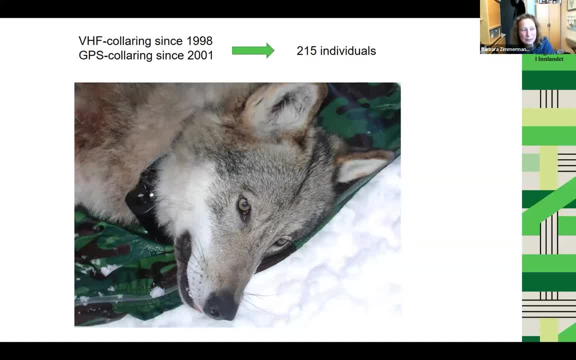 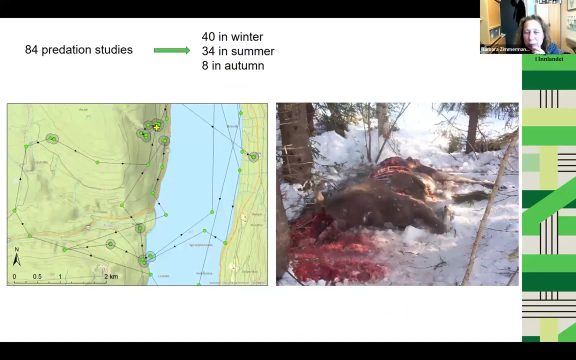 study the predation of wolves on wolves, because that was kind of one of the main um conflicts or or maybe let's say one of the first questions that were raised when wolves came back. it was like what, what impact will these wolves have on the on the most population? and so we started to do this predation studies, um where? 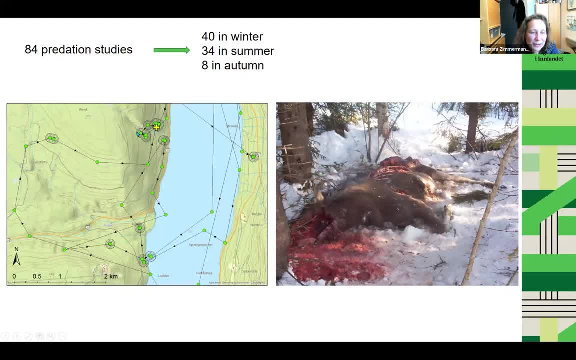 where we go into clusters of positions, uh, where, like the wolves, have spent several hours at the same place, and then we search those positions shortly after the wolf had been there, and then we try to see if we find uh, rests or like of carcasses or that the wolves had been killing and eating on, and so 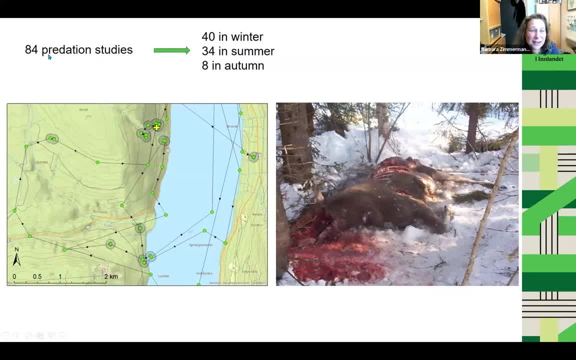 so far we have done 84 such studies in different seasons and, um, and actually sophia was doing one of those studies in summer study now this summer, and and when we do that over a certain time, a certain amount of weeks, then we can actually uh calculate the kill rate uh from this. so, in total, we have found 1426 carcasses and 80 of them were kind of- uh, killed by wolf, certainly, or probably killed by wolves. so they don't do that much scavenging. they do a little bit, but they mostly kill their own prey in our area. 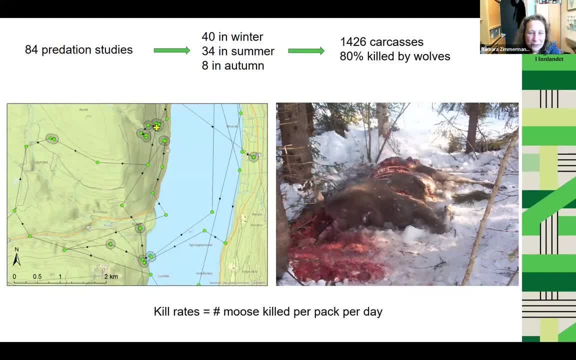 and so by calculating kill rates we can kind of do, then we can extrapolate for an entire year, so then we know how many moose an entire, an entire wolf pack kills every year. the kill rate in itself is not actually that interesting, it just says something. 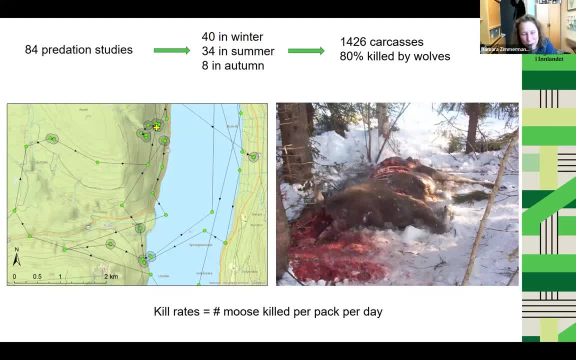 about how much wolves kill, but we for sure have to relate that to how many moose there are in the area. so if we find out that the wolves kill about 100 moose within a year, then it really matters if there are like 1000 moose in that territory. 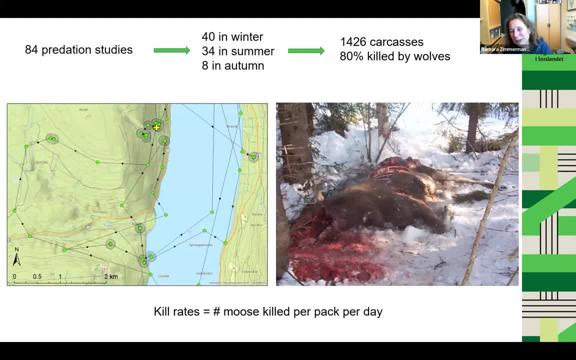 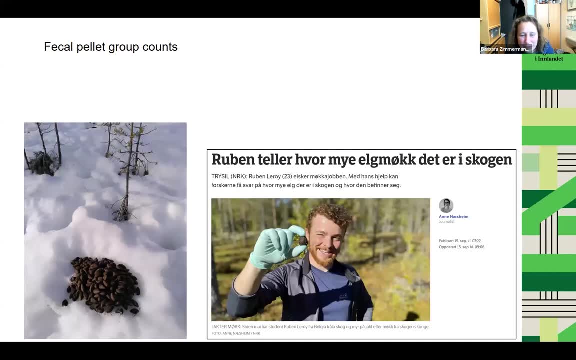 or only 200 moose in that territory. so we need to have a also numbers on how many moose there are and we do that with fecal pellet group counts here. you see, it was coming in the newspapers when we did one of those pellet counts. 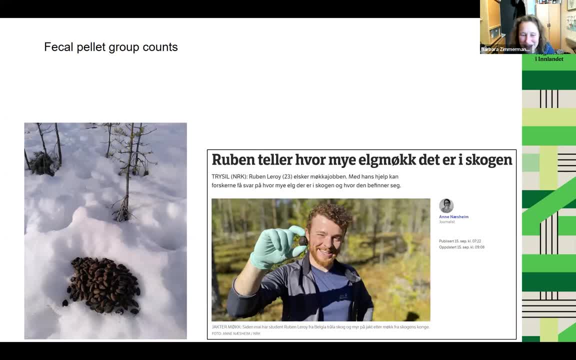 because the journalists think it's kind of funny that we go out and count all these moose piles in the forest. so it was kind of just a copy from a newspaper. yeah, I think. so with this fecal pellet group counts we can estimate the winter abundance of moose. 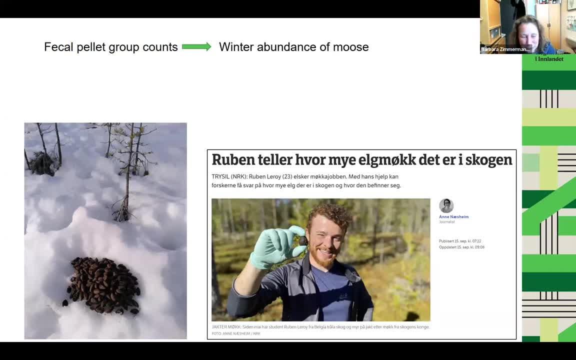 because we know the defecation rate. we know that moose poop about 14 times per day, and so we can kind of estimate winter abundance of moose if we then add all the moose that have been killed by wolves from our predation studies. 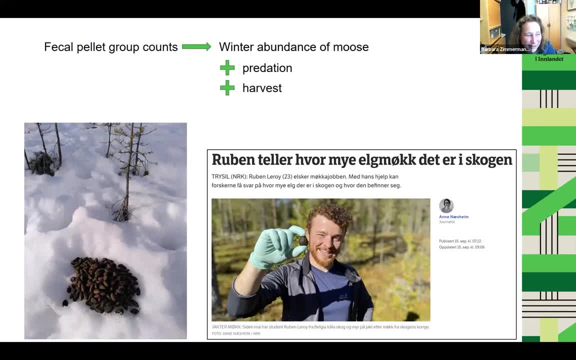 we know that and we add the hunting studies, so how many moose that have been killed during harvest and also have numbers on how many that were traffic killed, then we can kind of calculate how many moose we have after calving. and this is our kind of 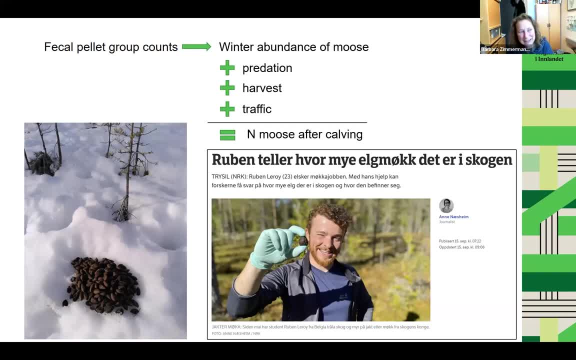 so this is the starting place: in 1st of June, it's just when the calving has happened or is happening during end of May, beginning of June. so this way we can calculate or estimate the number of moose that were available for a wolf pack. 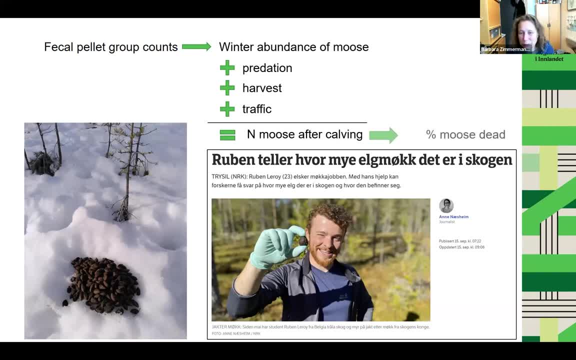 within the wolf territory after calving on the 1st of June, and then we would like to know how many or how large proportion of the moose that died, of these moose that were available, and again then to do that, that is kind of. 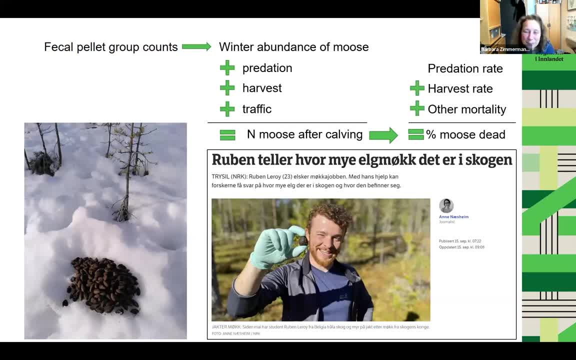 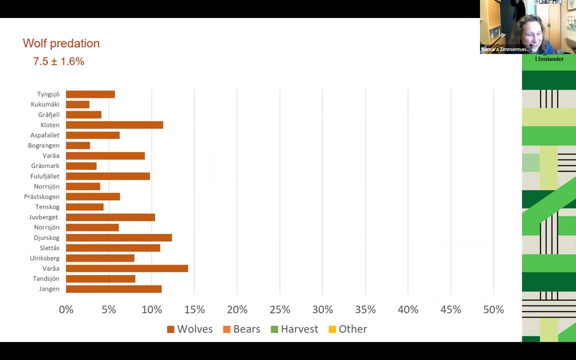 consists of the predation rate, so how large proportion that the wolves have taken and how large proportion that was taken by hunters and then other mortalities. so we have done this calculation and I here give you kind of the main results. but you can see here this long line with names. 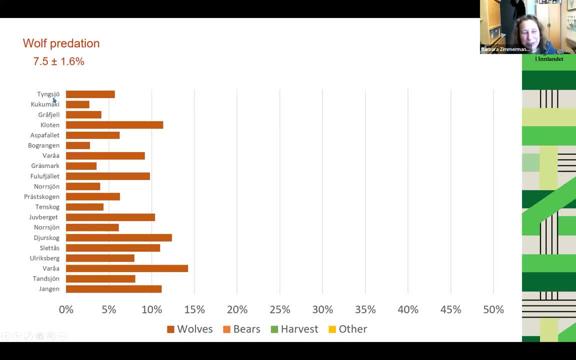 very strange looking names. these are different wolf territories and on the x-axis here you see the, the percentage, and so this is always the mortality. so how large proportion of the moose that had died here, for these orange bars are the wolf predation. so on average, 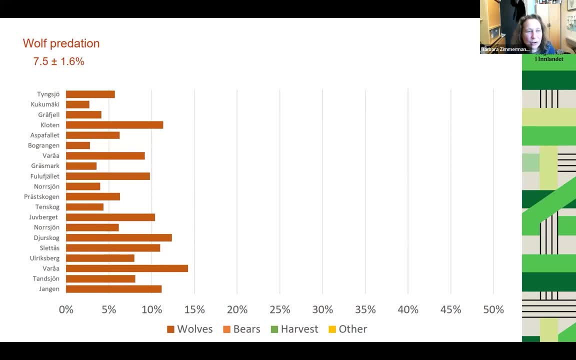 7.58% about of the moose that were in the territory by 1st of June died due to wolf predation. and you see there is quite some variation and I will come back to that variation later. and then in some of the territories we also have bears. 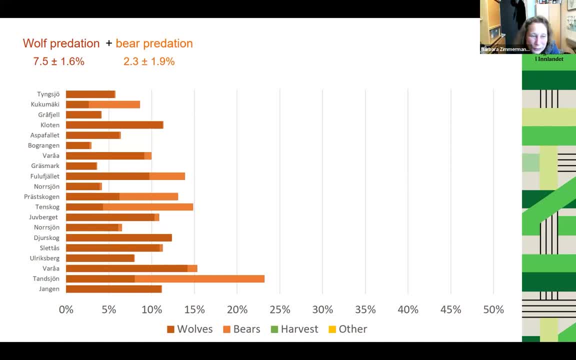 brown bears, or in most of them actually, but in some we have a lot and in others we have very few, and so the bear predation makes up about 2.3% on average, but you can see that in some areas the bear predation is even more important. 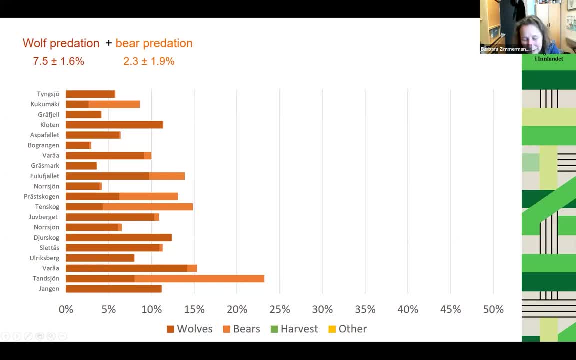 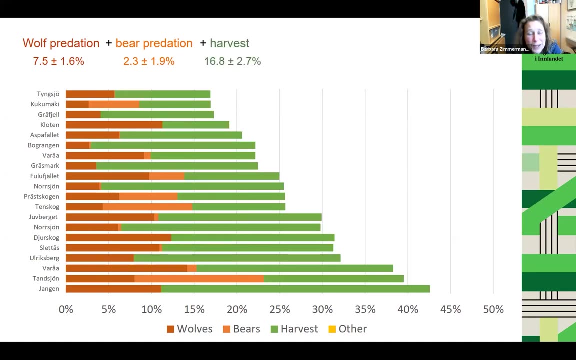 than the wolf predation bears. they kill newborn calves in the summer, just after calving, for about 3 to 5 weeks after calving, bears really like to pick those newborn calves. and then we have harvest. harvest makes up on average about 17%, so 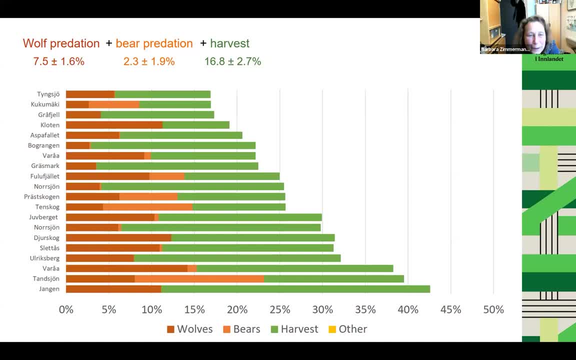 and again you can see there is some variation here, but it's about 17%. and then traffic and disease. together we have estimated on about 2.5%. we have very good number on traffic accidents, but we don't have good numbers on diseases. we have some numbers from: 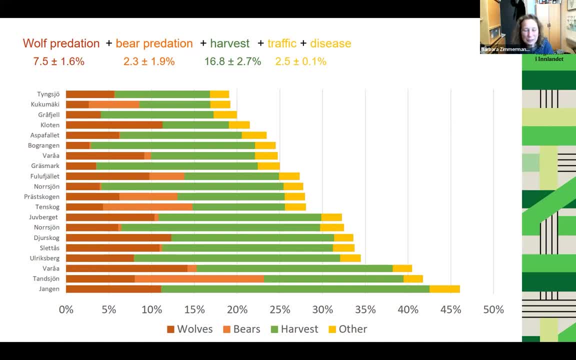 GPS collared moose, so that's why we can kind of know how much it makes up about. so if we sum this all together, the annual mortality that happens for moose is about 29%. so nearly one out of three moose die every year. can you see that? 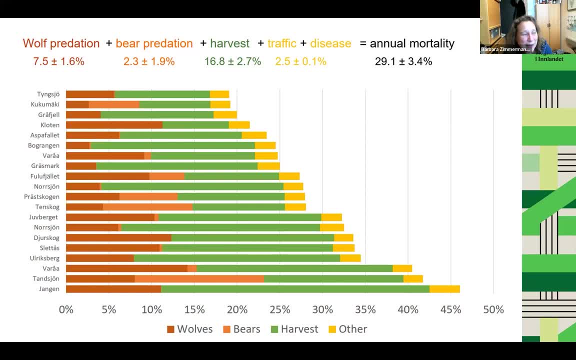 so and this number actually relates very well to what we know about the reproduction potential in moose. so moose like the moose population- if it was not regulated it would grow like with about 30% each year. so this 29% fits very well with. 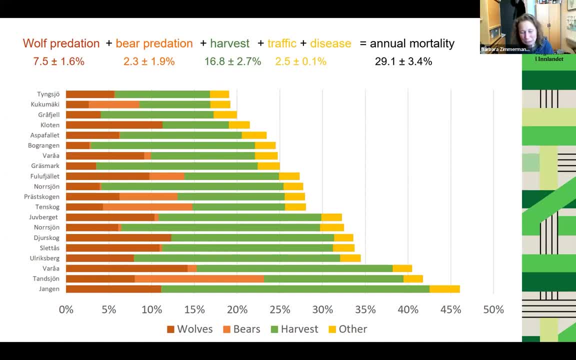 with the potential that the moose has to kind of reproduce and with the recruitment of moose every year. so but then, as you can see here, there is quite some variation in wolf predation, and so we have tried to find out what explains this variation in wolf predation. 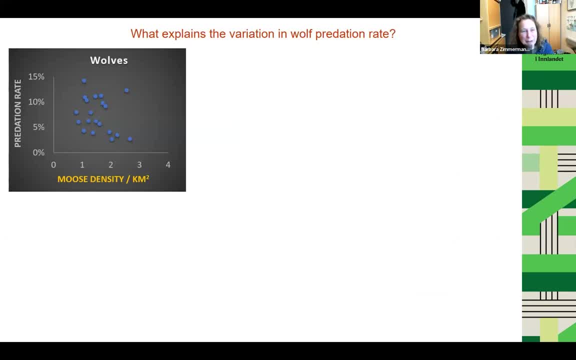 so we saw that one factor that might be important is moose density, but actually we don't find any relationship between moose density in the area and the predation rate. so moose density doesn't really make seem to make a big, a big, yeah- difference. but 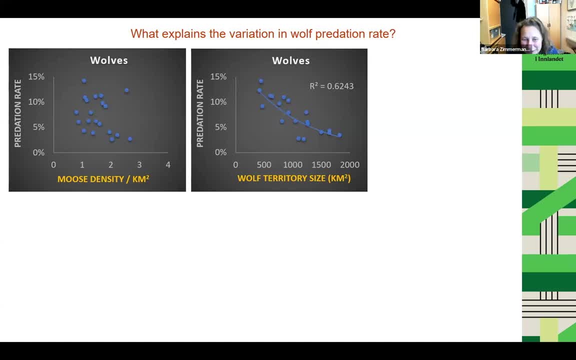 we see a clear relationship with wolf territory size. so in wolf territories that are very big we have very low predation rate on about 2%- 2.5%. but in small territories the predation rate can be very high. and why is that? yeah, that is because in small wolf. 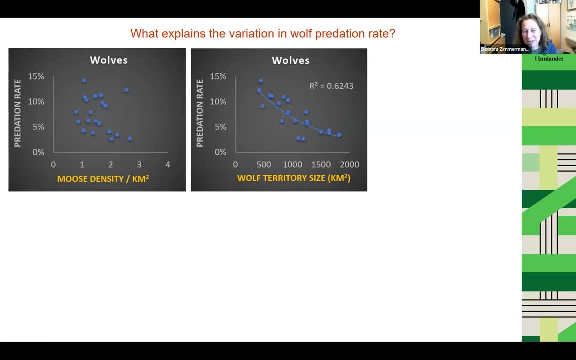 territories there are not that many moose. so actually moose abundance is the most important factor. so if we combine moose density and wolf territory size then we can get the moose abundance. so the number of moose it doesn't say no moose within territory, but it says the number of 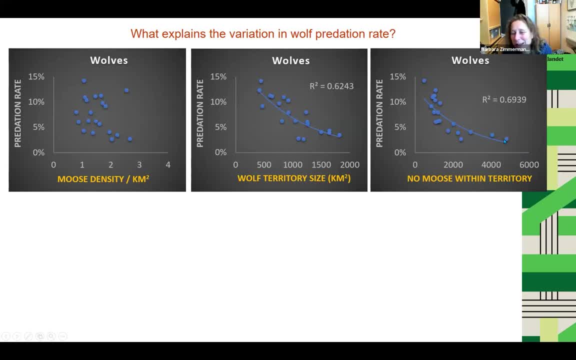 moose within the territory. so the number of moose within the territory, if there are many, then we have kind of a very low predation rate. but if you have few moose, which is kind of a combination of small wolf territories and small moose densities, 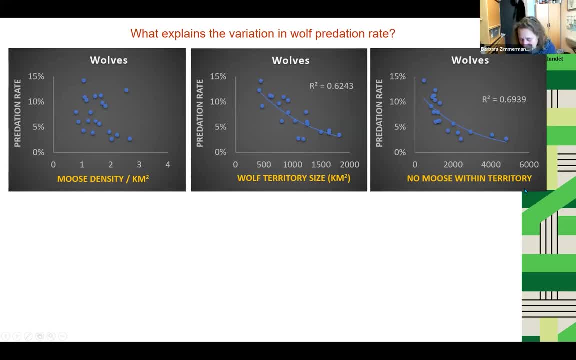 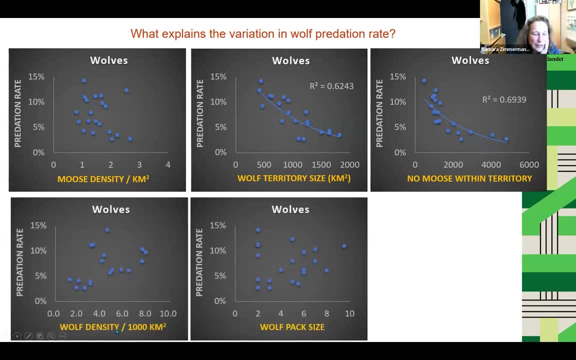 then we have a high predation rate, right? we also tested some other relationships. we were, for example, interested to see if there was a kind of a relationship with wolf density per or with the wolf pack size. so do big packs, or like large packs? do they have a higher? 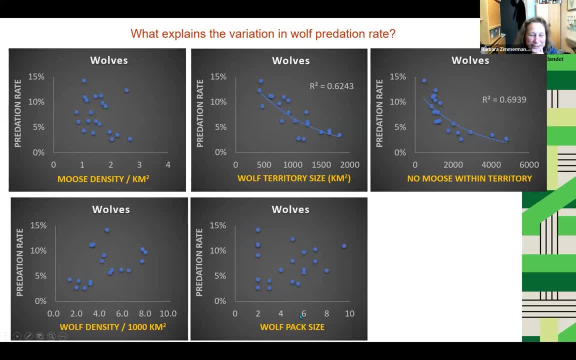 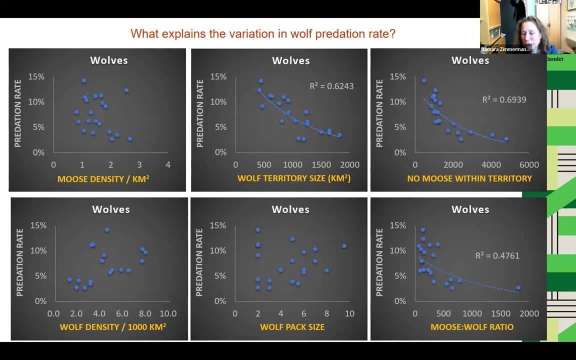 predation rate than small packs. but we don't actually see any any relationship for wolf density and wolf pack size. so even small packs can kill as many moose as large packs. but when we look at the moose to wolf ratio then we get a negative. 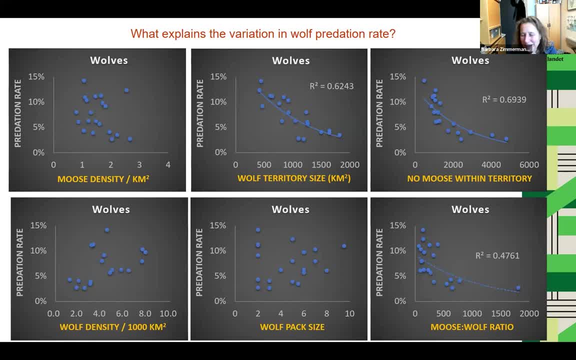 relationship here, but it's as you can see. there is kind of an outlier that is probably very influential for this relationship, so it's not very strong. so how many moose are per wolf? that is a better description than just only the wolf density itself. right harvest rate. 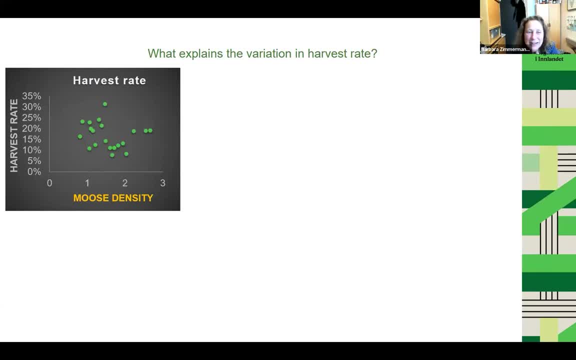 we also saw there was some variation in harvest rate, and so we also wanted to test what explains this variation. and first we did the same as with the wolf: we wanted to see if it depends on the moose density, because you would expect that maybe in areas with high moose, 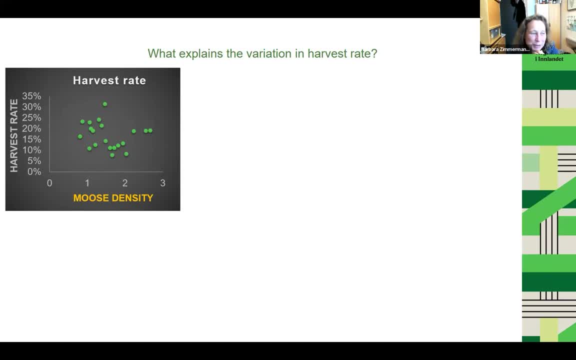 density, the harvest rate should be lower because the data maybe don't manage to kill as many as many moose, but actually we didn't find any relationship at all. so it was now not connected to moose density and I think that has to do with the fact that 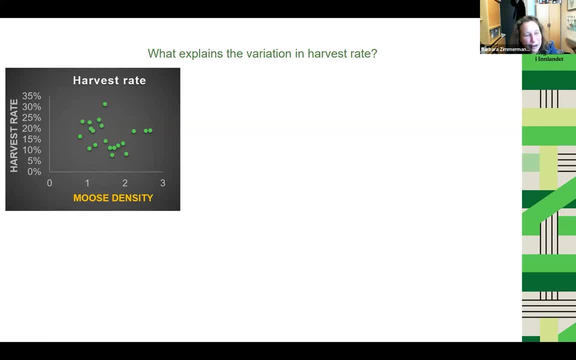 actually the moose harvest is the strongest regulating factor of the moose population, so we use harvest as a management tool to decide if we should have more moose or less moose, and so we cannot directly relate it to moose density, but we could say that way. 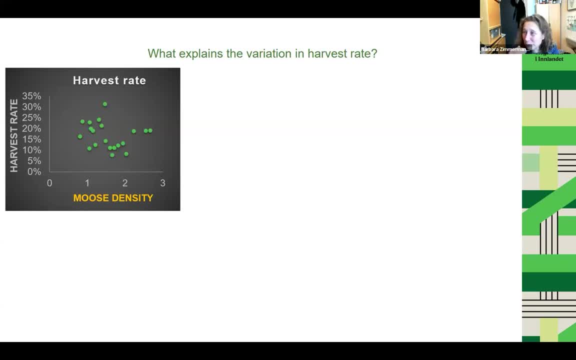 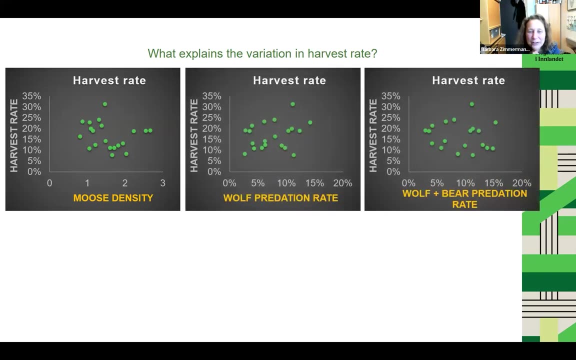 that when there are a lot of moose, then maybe we would like to reduce the moose population, but that again depends on the area and depends on forest and how, what the goals are for forestry, for example. so there are other factors that are important also. we didn't 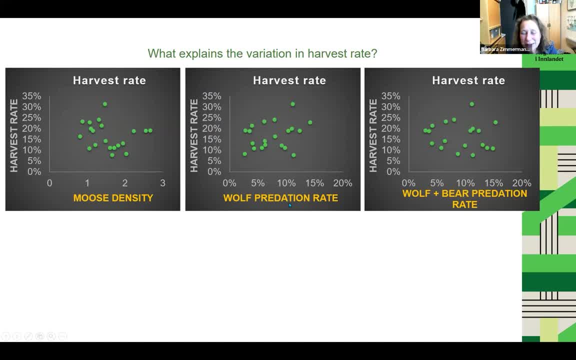 actually find any relationship between wolf predation rate and harvest rate. we thought that maybe there should be a negative relationship, so if wolves take a lot of moose then the harvest rate maybe should be lower. but actually we cannot find any relationship there, and also not if we add the bear predation. 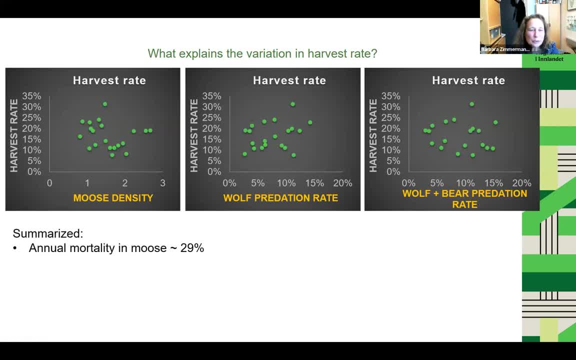 on top of it. so to summarize all of this, the annual mortality in moose was about 29%, estimated wolf predation rate about 8%. so you can see it makes up about one fourth of the total mortality. harvest rate is the double of the wolf predation rate. 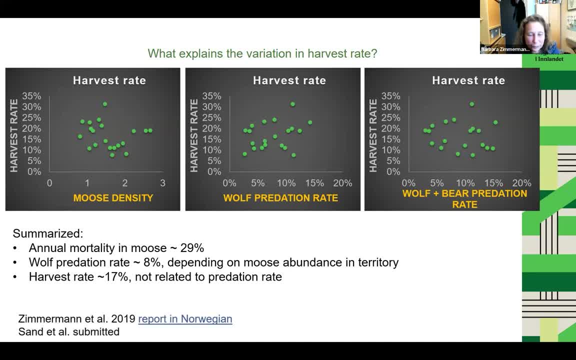 17% and it was not related to predation rate, and we have a report in norwegian that describes all this, but we have just now submitted the manuscript for peer review, where we also are presenting this results, so i hope you will be soon be able to read. 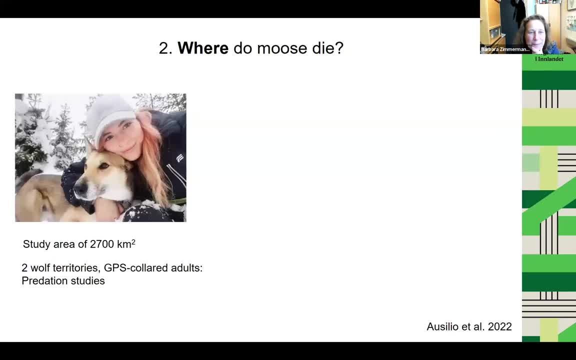 read them in a scientific journal. the second question: where do moose die? so for this i want to present you the work done by our phd student that we had during the last years, georgia ausilio. maybe some of you know her. she has been working a lot in our 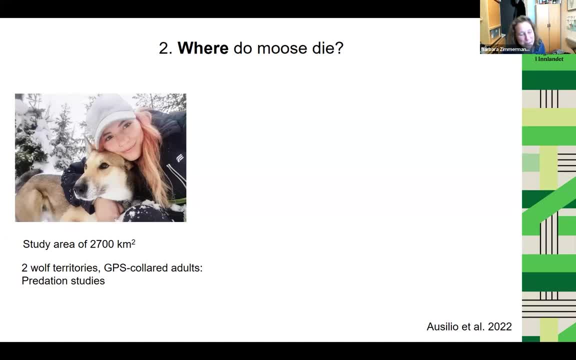 project that was called grenzewild border wildlife and she has looked into this question: where do moose die? she worked in a study area of 2700 square kilometers. it was a cross bordering study area that included areas of both norway and sweden. 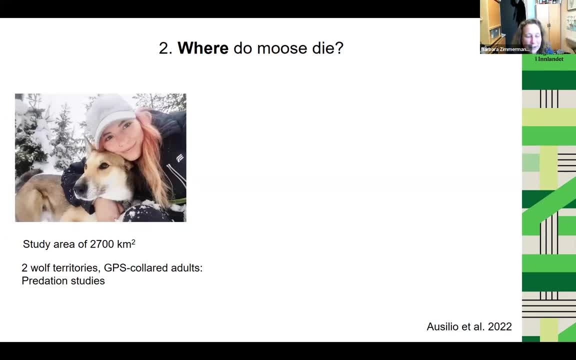 inside the area where we have wolves and we had gps collared wolves in that area, two wolf territories, and we did those predation studies and from those predation studies she used machine learning to predict all kill sites during autumn and winter based on the movement pattern. 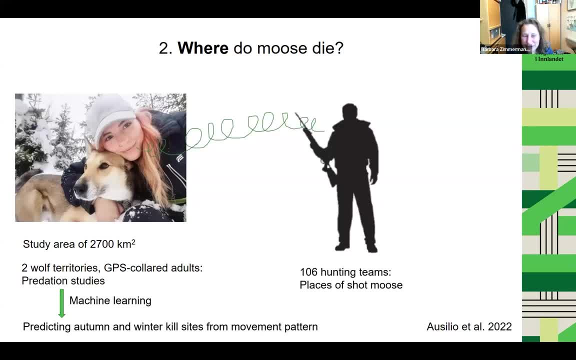 and then, in addition, she called. she called 106 hunting teams, all the hunting teams in that area, and asked them to give them the coordinates of where moose were shot. she did an excellent job to convince all the hunters to actually tell where they did shoot the moose. 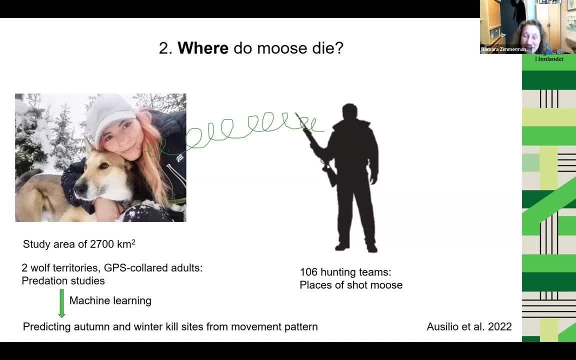 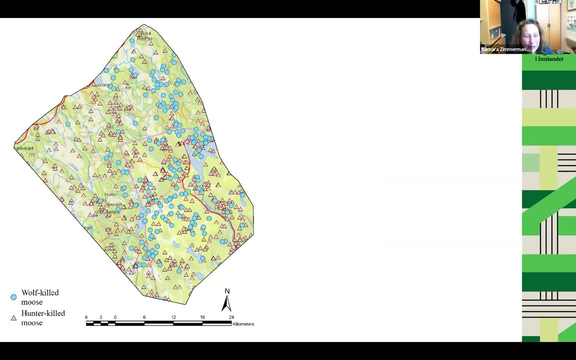 and so she has got a map for over two years that shows all those places and this is how the map looks like. so the blue circles are the wolf- killed moose based on the movement pattern and the predation studies that we've done, and the triangles are the hunter- killed moose. 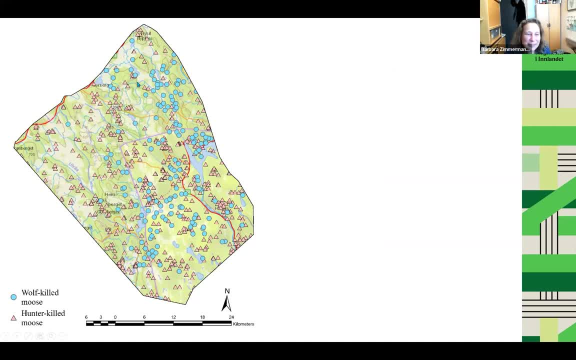 that were reported by the hunters and, as you already can see, there is some difference between how the blue circles are distributed and how the triangles are distributed. triangles are more or less all over the place, whereas the blue circles are a bit more concentrated in some areas, and 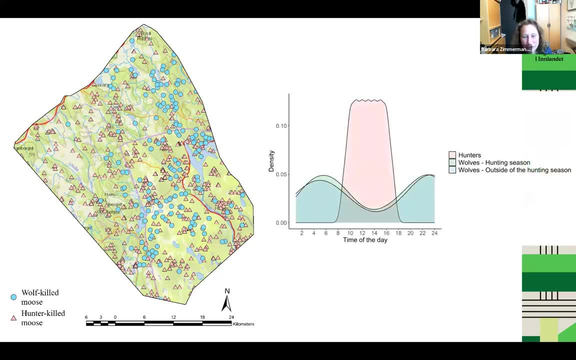 so what she did next, and she also looked into the temporal effect. so when is the risk highest to die in harvest? that is for sure during the daytime, during the hunting season, but when it comes to wolf predation, that's mostly during night time, and then again. 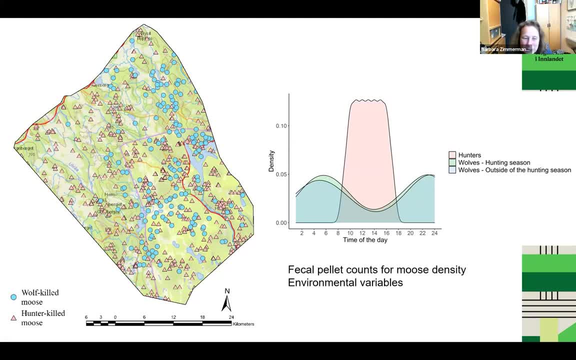 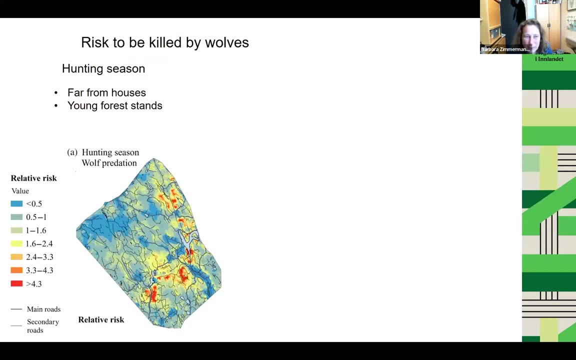 we did these fecal pellet counts to estimate the moose densities in the study area, and she also used a lot of environmental variables to describe the habitat, and so what she wanted to describe is what is the habitat for the moose? so she did this for 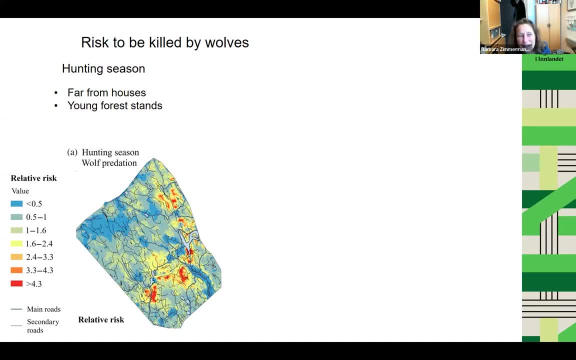 wolves and hunters separately. so risk to be killed by wolves during the hunting season the risk was highest far from houses and in young forest dens. and you can see that on this map from blue to red: blue is low risk and red is very high risk. and then after the hunting season, the risk to be killed by wolves was highest close to roads- which maybe you think is a bit surprising, and I will explain you why later- but also in young forest dens. so why close to roads? this is because moose- in the winter they migrate. 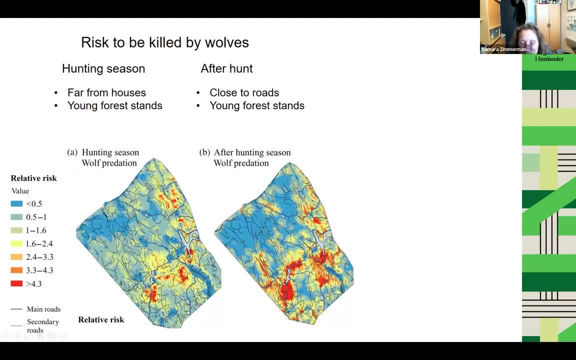 from summer areas down to the valley- and here you can see one of these valleys here and one of the valleys here. they migrate down into those valleys because there is less snow and more food available, and so the wolves, they actually follow after the moose or use those areas. 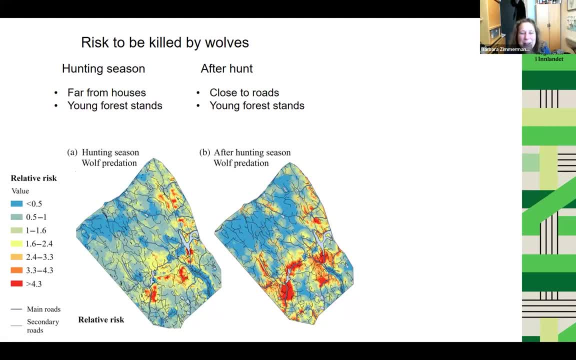 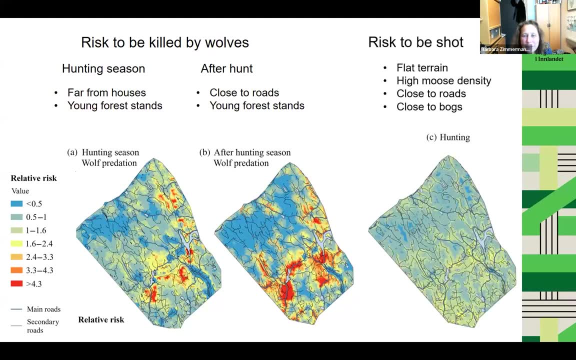 I mean, they don't really follow after, but they use those areas more down in the valley and that's why the risk is higher to be killed by wolves in those areas. the risk to be shot is kind of here. you can see from the map already, from the colors, it's kind of more. 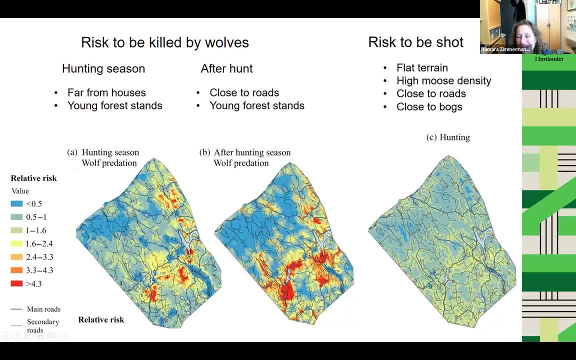 even distributed all over the landscape, so you don't have this dark red and dark blue, but it's more kind of there is kind of a risk in this. yeah, here you can see one to 2.4. so it's kind of the risk is kind of more intermediate. 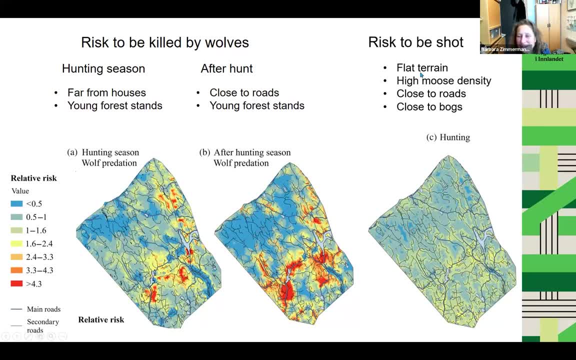 but it's all over the place and it's a higher risk in flat terrain at places where moose density is high, close to roads and also close to bogs, which also means it's kind of more open areas. and then the next question is: how can you survive in such a landscape of risk? 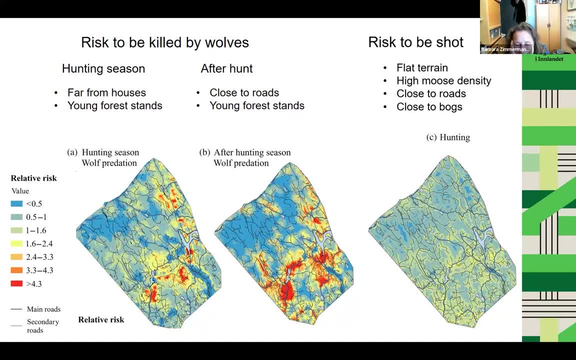 so if you're a moose and you have to navigate in this landscape, and it even changes from between day and night, so you know, this is more kind of what happens, how the risks look like during night, and this is more what it looks like during day time. 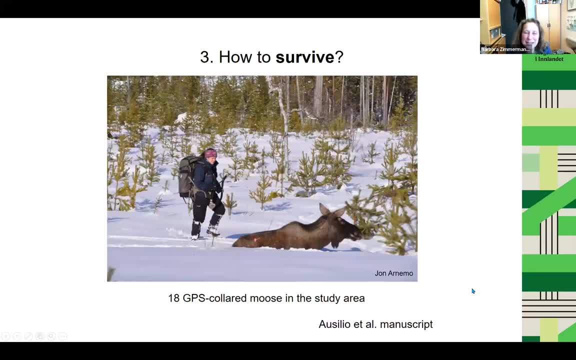 during the hunting season. so how would you navigate in this? so this is the next question: and how to survive? so we had 18 GPS colored moose in this study area. actually this here: it says Auxilio et al manuscript, but it has just been accepted. 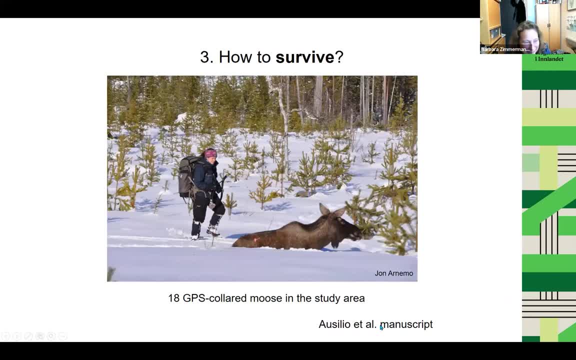 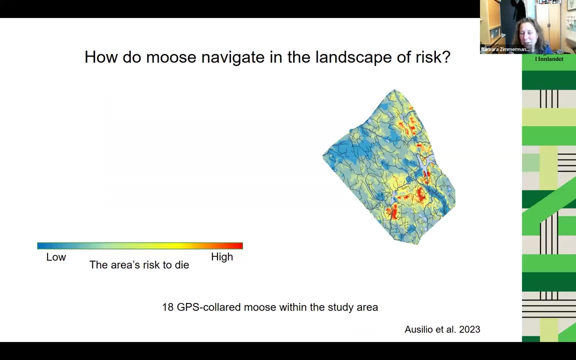 for publication. so it will be Auxilio et al 2023 and will be published in ecology and evolution, so it will be out anytime now, maybe this week, maybe next week. you can read the manuscript there. so she looked into the habitat use of the moose. 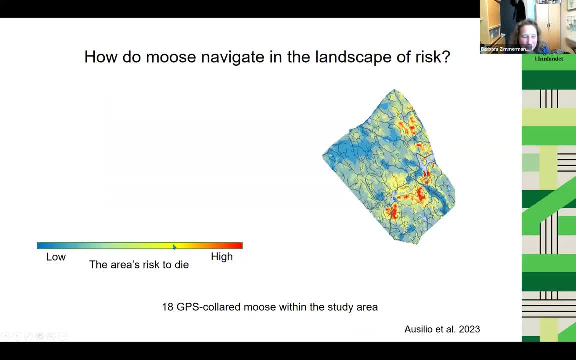 in this landscape of risk and again. so we have this gradient from low risk blue to high risk red, and sorry, that was wrong. and so she looked at the moose selection for a given area. so would they like go for low risk areas or high risk areas? 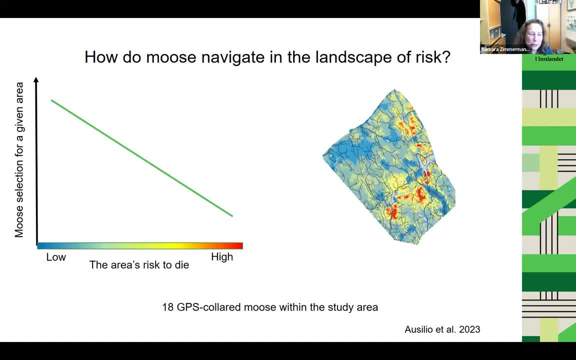 and for sure. we would expect something like this: that moose would select mostly low risk areas in those times when they are risky and high risk areas would be avoided. so low selection for high risk areas. but it is not that easy. we have to take into account. 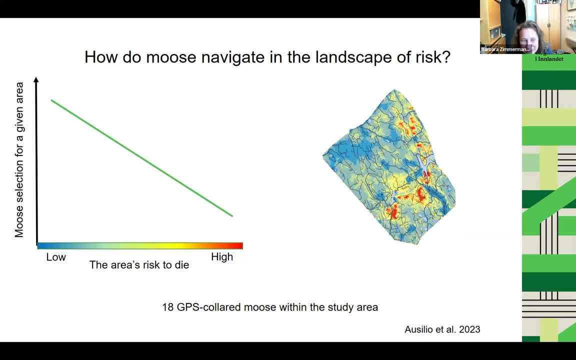 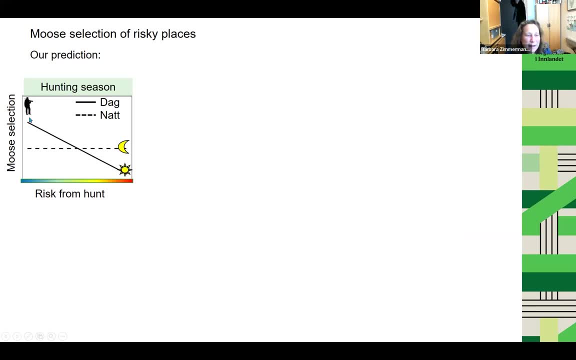 the time of day and also the reason to die. so, for example, we would predict that when it comes to the hunting season they should select areas with low hunting risk and they should avoid areas with high hunting risk during daytime, but during nighttime they shouldn't really bother about it at all. 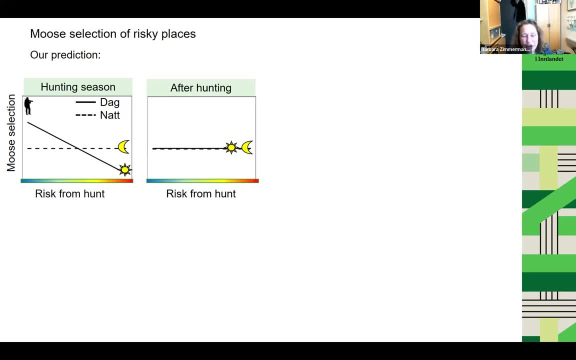 and then after the hunting season, we would think that they don't really bother at all about hunting risk at all, because there are no hunters out there anymore, independent of day and night. when it comes to wolves, we would expect this negative relationship with moose selection only during nighttime. 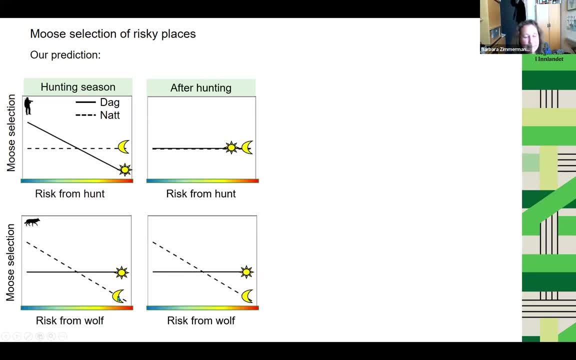 so avoiding areas of high wolf risk in the night, but during daytime we wouldn't expect any difference between risky places, and it doesn't really matter if it's during hunting season or after hunting season. we would expect the same pattern. so what did Georgia find? actually, she found as we had predicted. 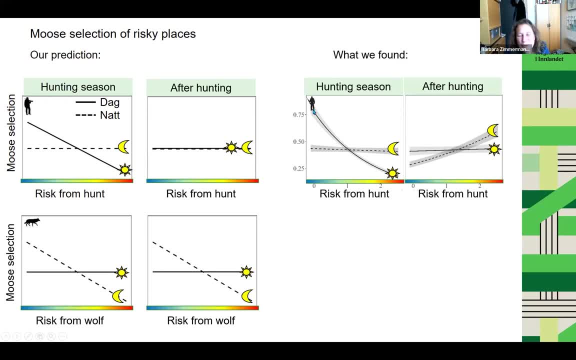 more or less when it comes to hunting. so the moose were really avoiding those areas during daytime that had high hunting risk. so they are smart animals but and in the nighttime they didn't really bother, and after the hunting season they didn't bother during daytime and they even used a bit more time. 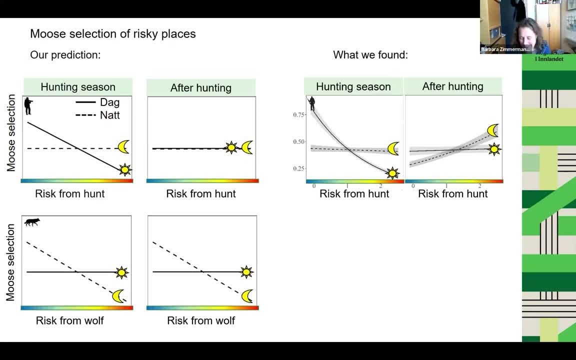 in those areas that would have had high hunting risk during daytime, and when it comes to wolves there, actually it was very surprising. it was exactly the opposite of what was expected. so moose were actually trying to select for areas with high wolf risk, independent of time of day. 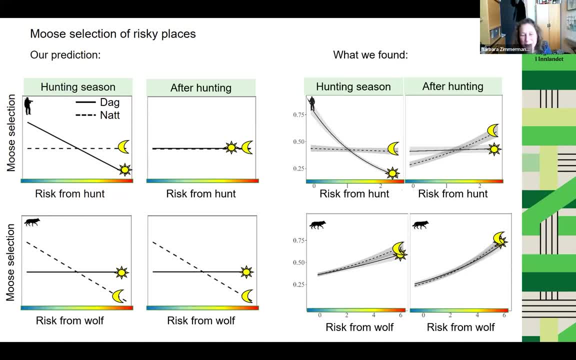 and time and season, so that was really really interesting. and so then the question is: what's going on here? yeah, I don't really remember what was really the important factor that explained the landscape of risk. when it comes to wolves, young forest stents are really important. 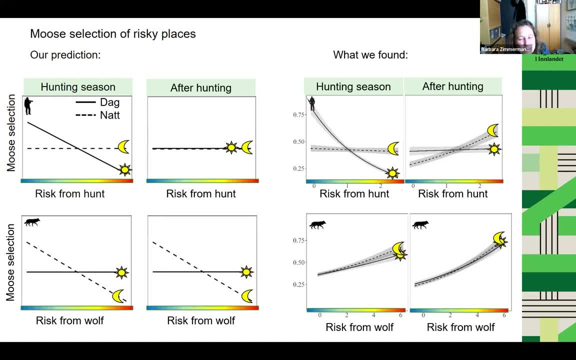 they have a high risk and so probably for the moose it is kind of a trade off. the moose has to decide between food and the risk of being taken by wolves. so if you have maybe 1000 moose within one wolf territory, the risk that 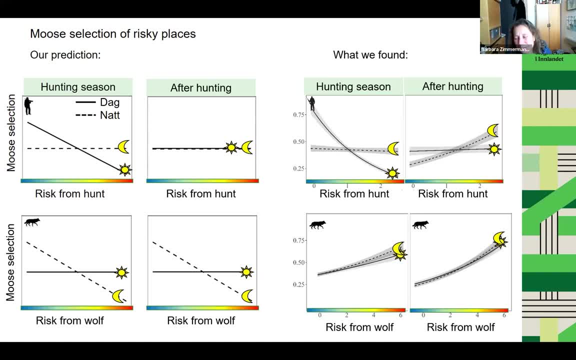 it's just me. me as a moose that is going to be taken by a wolf is kind of quite low, so then it's maybe worth actually to take the risk and rather fill up the belly with a lot of food and with that also being more able to, for example. 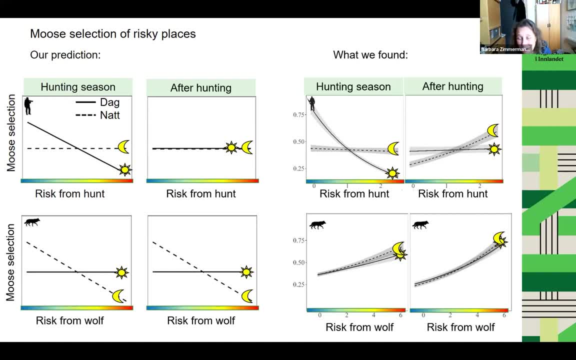 fight against a wolf attack. so there is probably this trade off and another explanation is also that moose maybe still is kind of naive to the to wolves. the naivety hypothesis is really interesting. we have been publishing several papers on that where we kind of think that the moose 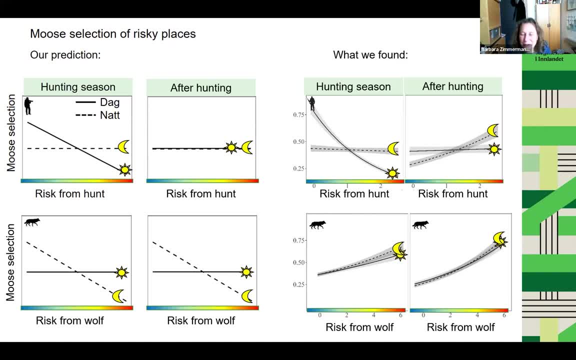 still is not really, doesn't really have the good predator behaviour that would be necessary to avoid wolf predation. and this can have several reasons, maybe because it has just kind of it hasn't really evolved it yet. but it can also have a connection with the way 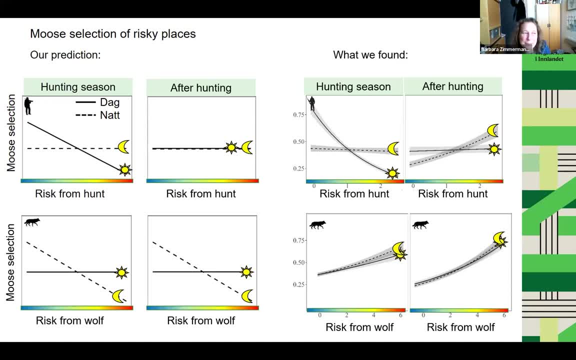 how moose are hunted. in Scandinavia we use those hunting dogs, the moose, moose hunting dogs that are kind of a little copy of a wolf. what they do is they are usually loose and they try to find a moose. and when they find one, 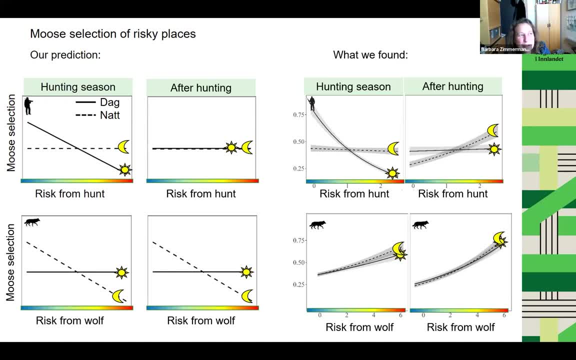 they start barking, and the moose should do what is best against the wolf attack. it usually stands its ground and tries to defend the call, and so what then might happen is that actually those moose are easier, more easily shot by the hunters, so there might actually have been. 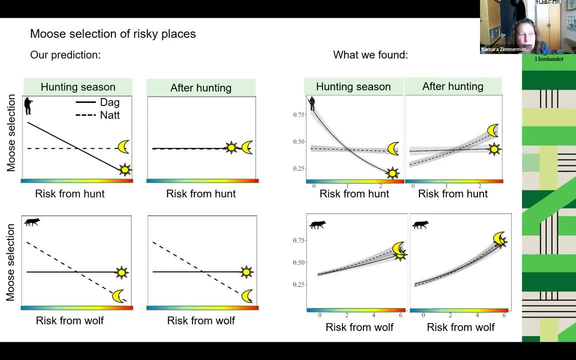 a selection towards moose that do the wrong thing. when it comes to wolves- and those are the moose that are running away- they are easy to be attacked by wolves, but they are harder to shoot for hunters, so my last chapter was about food, forestry, weather. 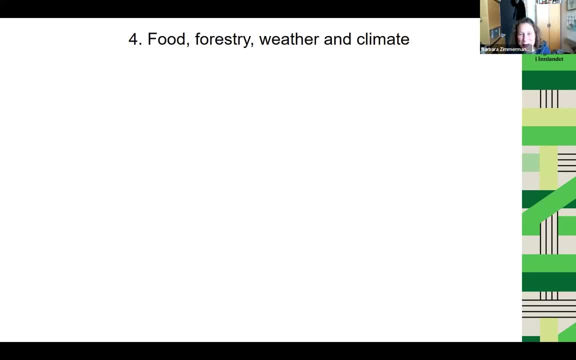 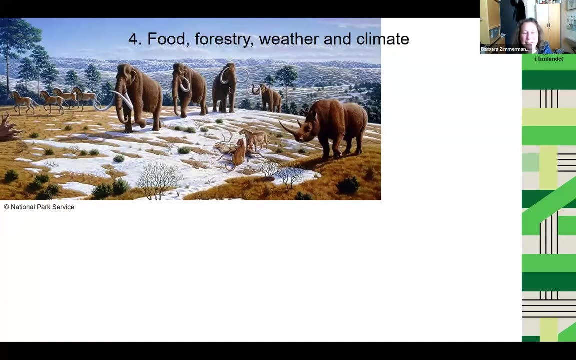 and climate, these complex interactions of how climate affects moose in in different indirect ways. for this we have to maybe go back to 10,000 years and see a little bit how Scandinavia might have looked like after ice age. we know that there has been. 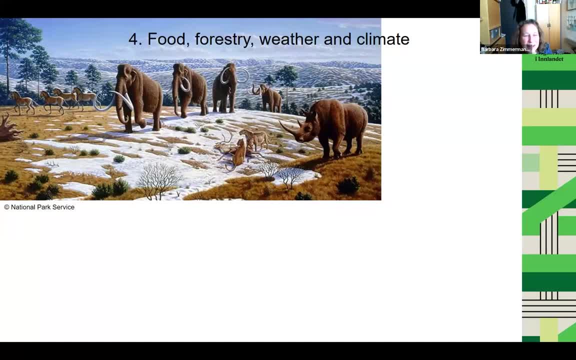 quite a different megafauna in these years and the porrel forest looked more like this, very open, a bit more like maybe you are used to in Hungary: big steps with a lot of grazers and some trees. but, as you all know, this megafauna- 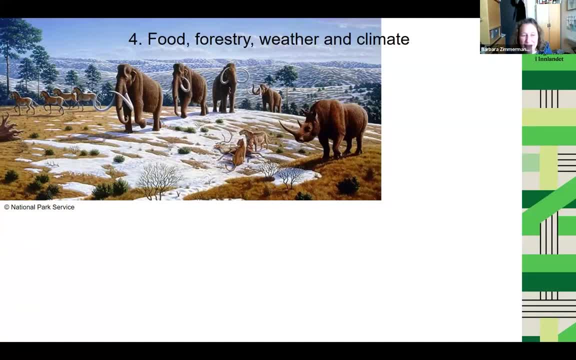 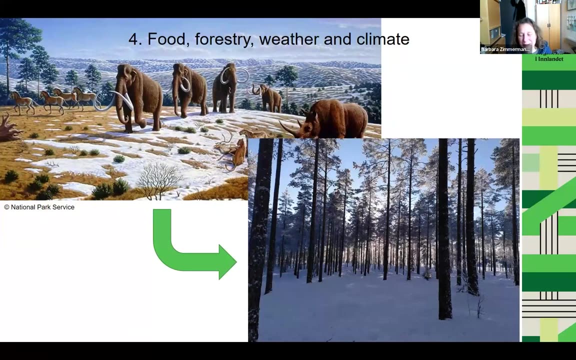 has been is gone. still don't really know why, but probably a combination of both hunt and climate change. but today the landscape looks like this: we have a production forest with very even aged stands. I have already been telling you about this: clear cutting practices and this makes very even aged. 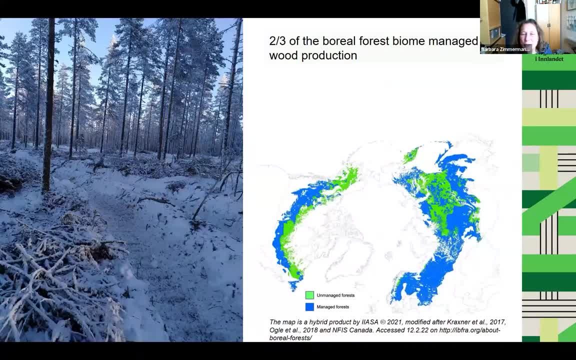 stands all over, and so two thirds of the porrel forest biome that we have like around the north pole, is actually managed for wood production. you can see that from this map here. it shows in blue all the managed porrel forest and in green it shows the unmanaged forest. 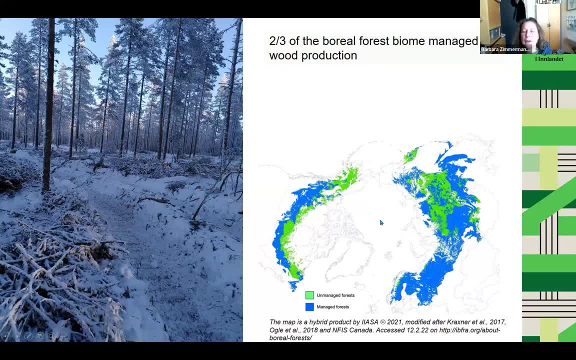 here is Scandinavia. the north pole will be here. most of the porrel forest is managed and actually, when you look at the global production, the porrel forest makes up 33% of all lumber and 25% of all paper produced, so it is a very important. 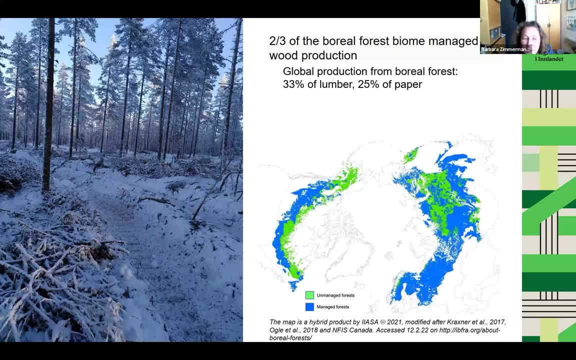 economically very, very important ecosystem or biome, and actually in Scandinavia 90%. you can see there is very little green, the most of it is blue. 90% of the Scandinavian porrel forest are managed, and when I say managed I mean that we harvest them. 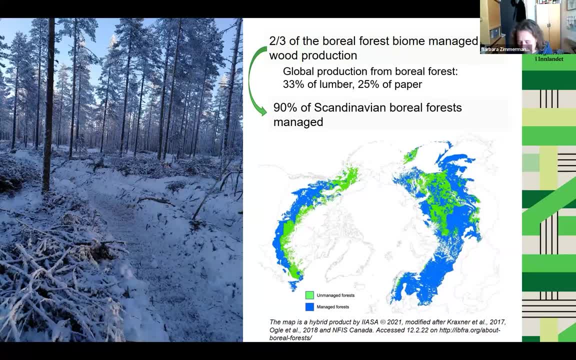 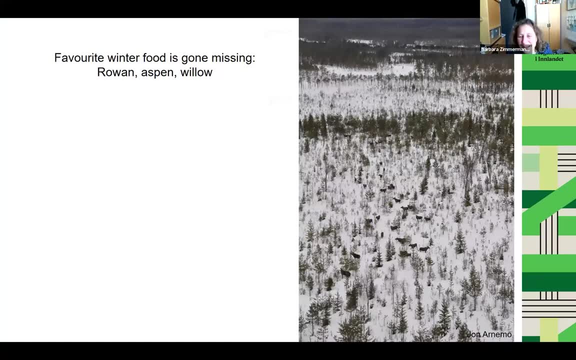 we make these even aged stands and we increase the productivity, and so this has, for sure, strong impacts. the favourite winter food in this managed forest is now missing moose. they don't actually like that much to eat these pine trees, but because there is nothing else left. 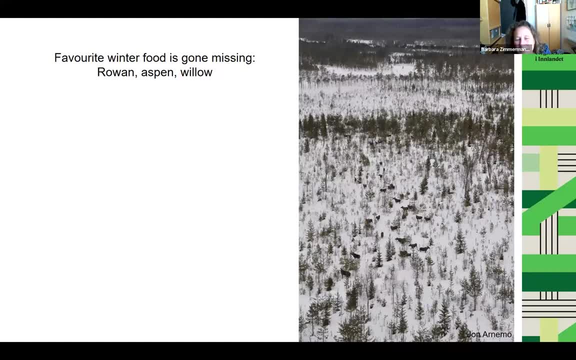 that's what they do. rowan, aspen and willow are the preferred species for moose in the winter, but the forestry doesn't favour these species and also the moose population has increased a lot, so wherever those species exist, they are usually browsed. so they don't anymore. have like large trees because the moose don't allow them to grow up. they will be. they are cropped every year just above the snow level. so this, the consequence of that is that moose have to feed on other stuff that they don't like. 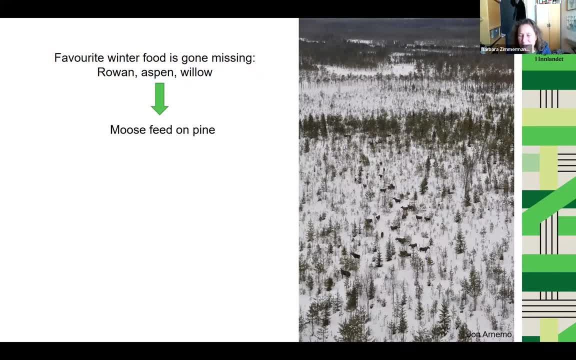 that much. they eat a bit of birch, but they don't like that, like birch that much neither. so they eat a lot. on pine, and pine, for sure, is not planted and produced for moose forage, but it's produced because the forest owner would like to have a lot of. 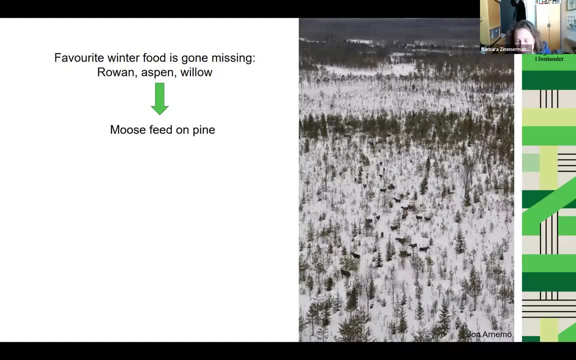 timber in 60, 70, 80 or 100 years from now. so then we get into this conflict between forestry and moose harvest and also conservation, because not only moose would profit from rowan, aspen and willow, but a lot of other species. 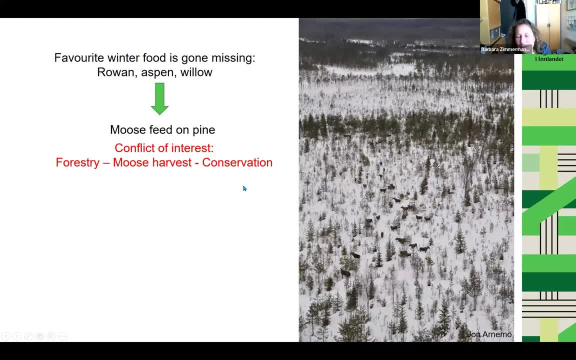 also couldn't. actually would like birds and insects would have much more. yeah, we would have a higher biodiversity if we had like more of the of the seedless forests. so we are studying. we have a project that just started that looks into how is this conflict affected by climate change? 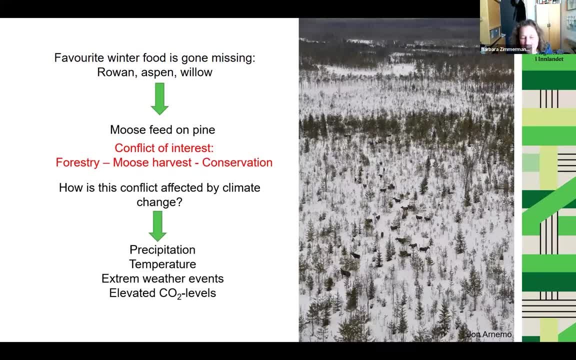 and we look into precipitation and temperature and also extreme weather events and also the elevated co2 levels that have kind of fertilizing effect on the forest. so those are, this taiga climate project, and then we also we have a project that we are going to finish up. 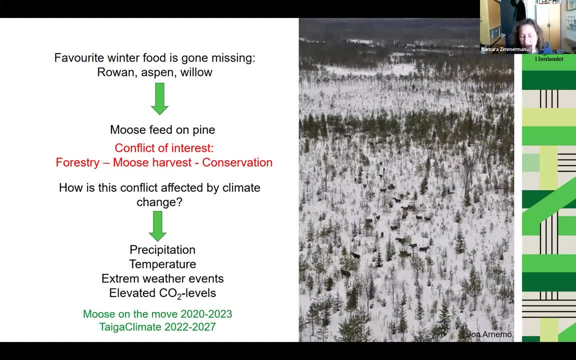 now that is called moose on the move, where we are looking into some of those things and where we have colored- yeah, the snow, sorry, i forgot the snow, but the snow is important here- where we, where we also look into into these things. so, for moose on the move, we 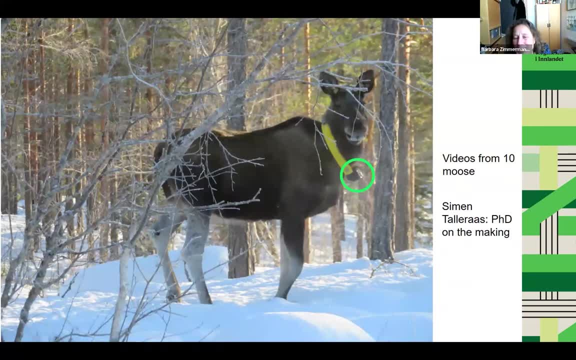 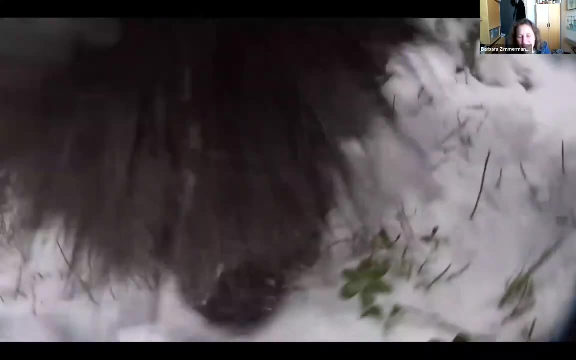 had like used video cameras on colors for moose and we have a phd student now that looks through all those videos- and we did that to see what they eat. for example, here you can see a moose that is eating on the blueberry that is covered by snow, so not the berries. 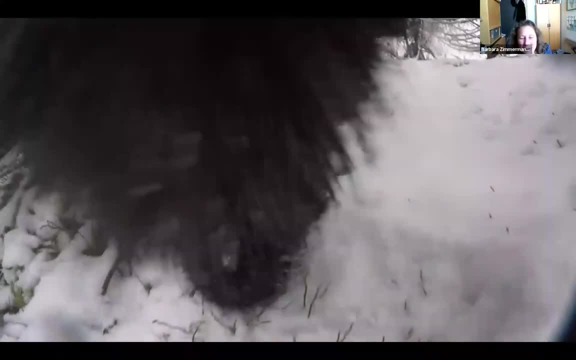 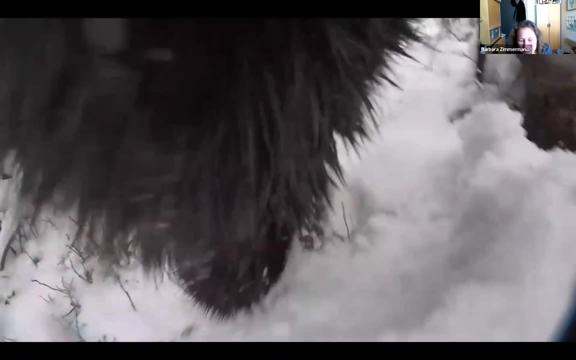 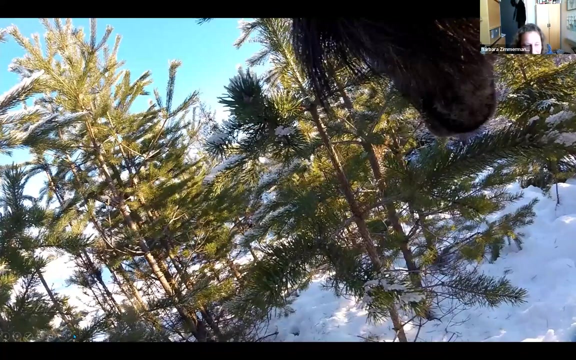 themselves, but the blueberries stems, so the so, as long as it's possible to eat this, they would actually like to eat this. this is kind of their favorite food, but when there is too much snow they will go over to eating pine. you can see here and. 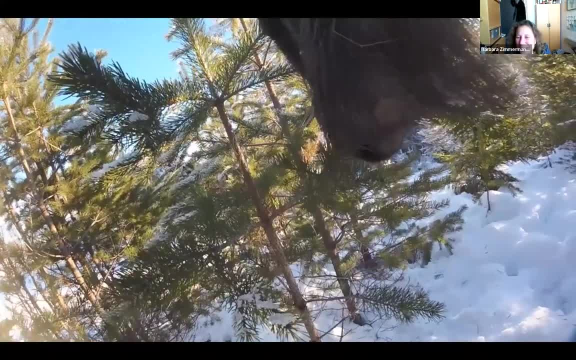 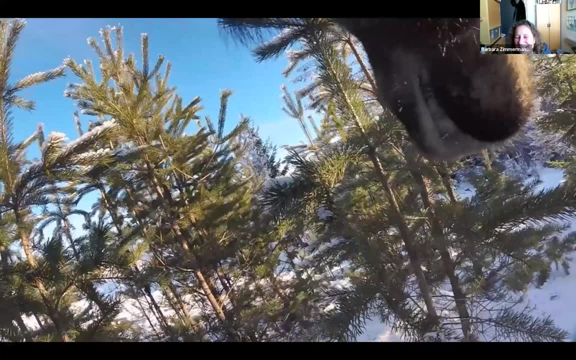 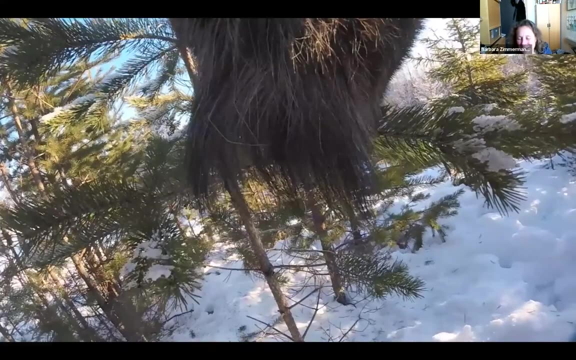 you see they are. i mean they eat it but it's not kind of. yeah, they probably have to be a bit careful when eating it because it's kind of sticky um, but for sure this can make big damage for forestry. so this is one of the one of the main issues we have in the forest. 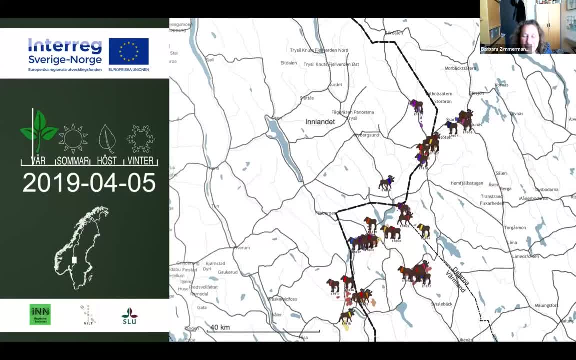 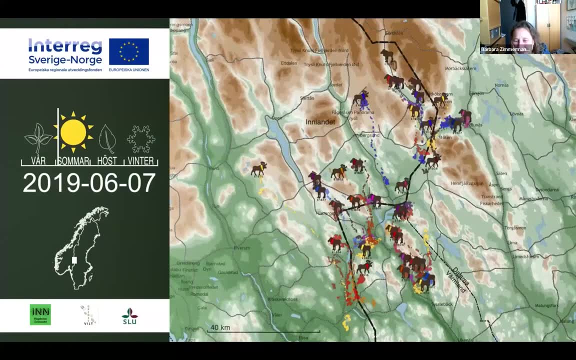 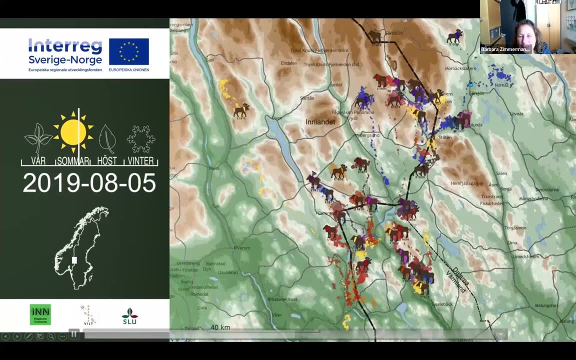 um, and this happens mostly in the winter areas. here it's kind of an animation of the moose that we had colored during our projects and you can see now in the summer they kind of distribute a bit more throughout the landscape, these different moose, and then in 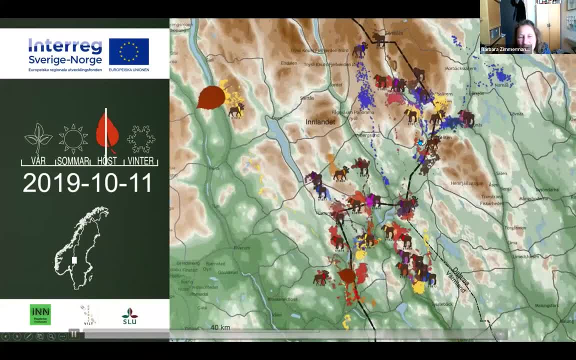 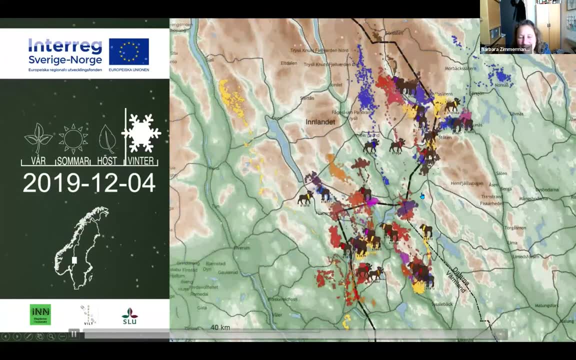 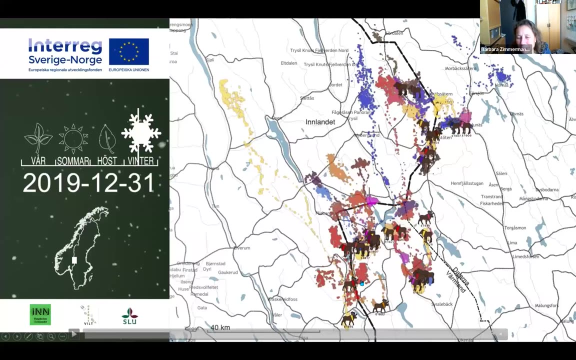 the fall our harvest has started. now they are still keeping in the summer areas and and now the snow is coming and they are moving back into their wintering areas and that's where we have a lot of this damage on pine and we have the problem with the forestry. 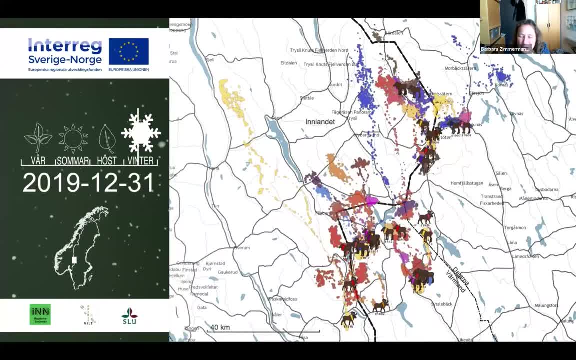 and for sure. this becomes a challenge because the ones that the ones living in these areas here where the moose concentrate in the winter, they have a lot of damage in the forest- but the ones that are living in the summer areas here where the moose had been. 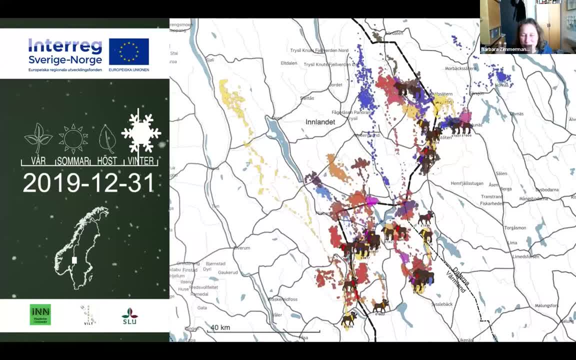 they have just only the harvest of moose, so they have kind of only the positive side of the moose and um, and so there is, there is this conflict of interest between the different landowners, and this is especially complicated when you have a national border, which is this black line here. 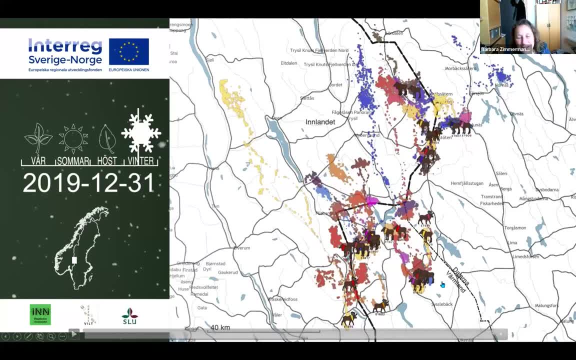 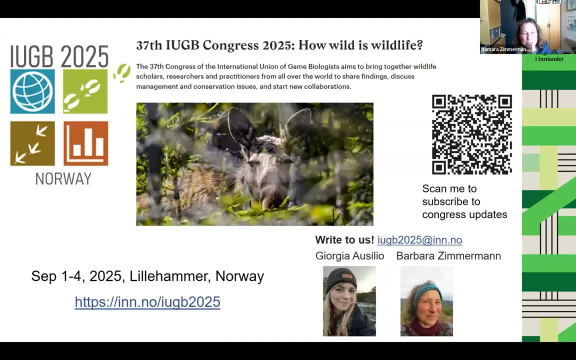 with Sweden on one side and Norway on the other side. but that would be a totally different talk and we won't have time to go into that now. so i'm more or less done with my talk. i only want to tell you quickly that we are going to host. 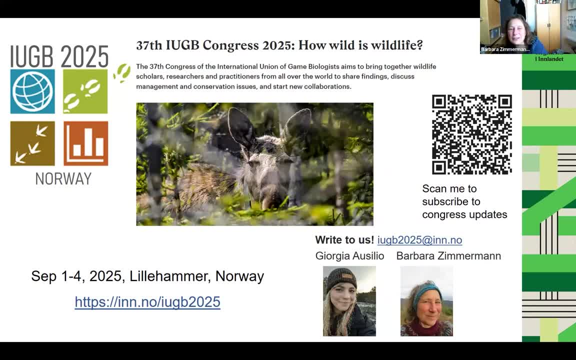 a big wildlife conference in Norway in 2025 with the main title: how wild is wildlife? it's a collaboration between IUGB and also the nordic congress of wildlife and also euro memos, and we will have this wildlife congress in Lillehammer in 2025. 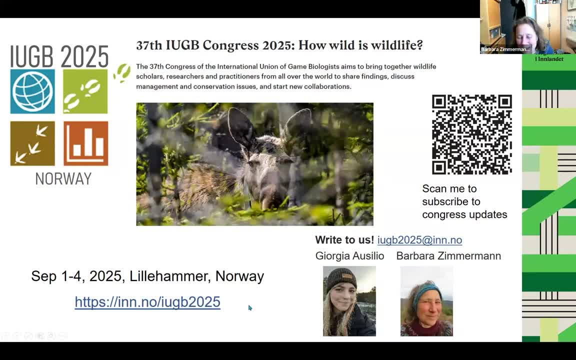 september 1 to 4, so please reserve the date. we will soon come out with a newsletter. you can subscribe to the newsletter um on our webpage or by scanning this qr code, and then you will get more information from us. so looking forward to see you in Lillehammer. 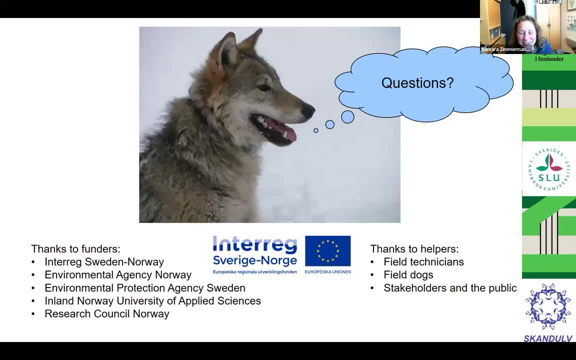 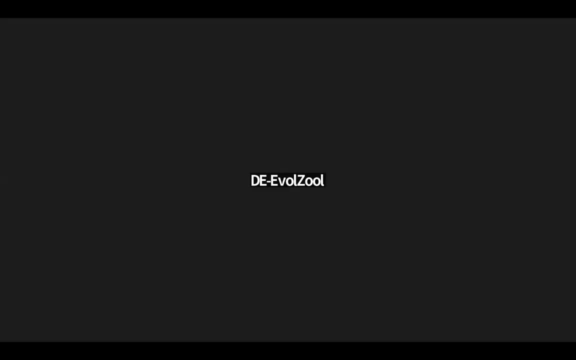 in two years from now. yes, are there any questions? do we have time for that? maybe not. uh, maybe you have a few minutes left. yes, we have seven minutes left, so please let me know if you have any any questions. yeah, we are waiting for questions, and everybody. 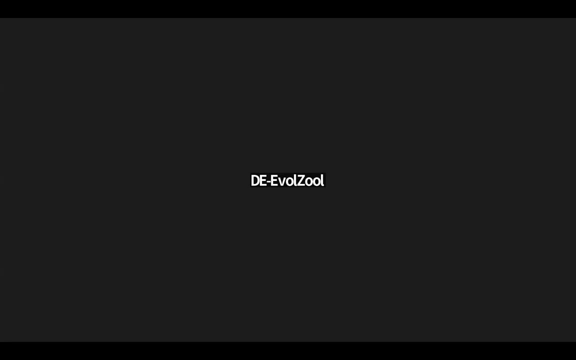 you can write your questions in the chat if you don't want to or you can't use your microphone. no, everybody happy. yeah, everybody happy. yeah. thank you, Barbara, it was a wonderful presentation. um, yeah, and for the participants, you can re-watch the seminar on our youtube channel. 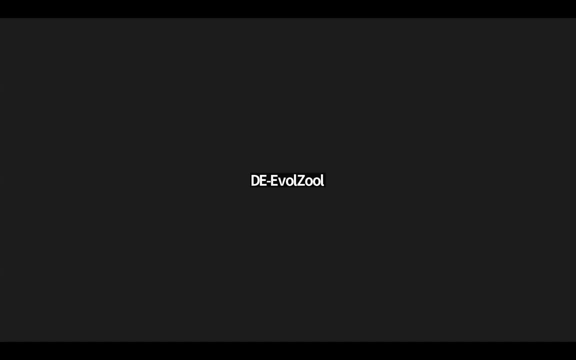 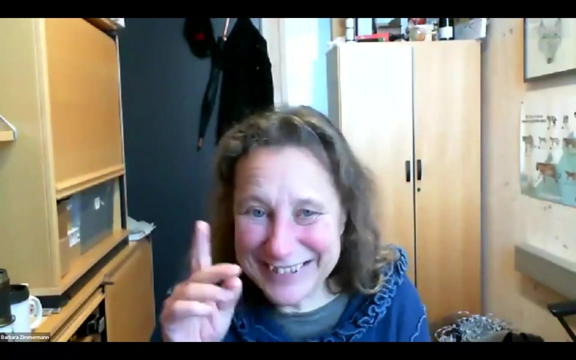 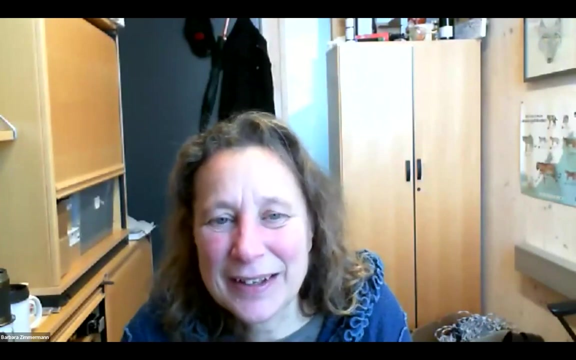 later or if a friend couldn't be here. thank you, Barbara very much, it was really exciting. um, and oh, there was a question coming in. ah, yes, yes, is there a significant competition with smaller mesoherbivores? um, that's an interesting question. actually, we don't know we have. 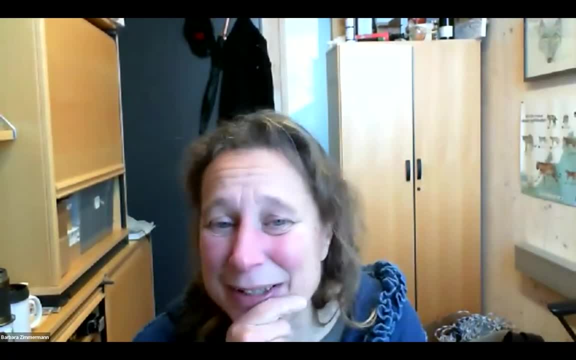 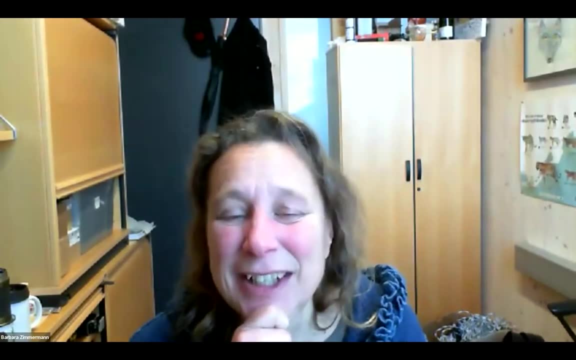 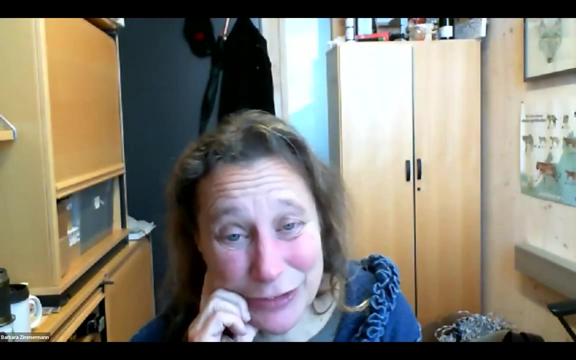 a colleague of mine is, has been working a little bit on this um, because the main species in mind here is the hare, the mountain hare. we have mountain hares here, um, and so there might be some competition there. and also we have, um, three students, uh, master students. 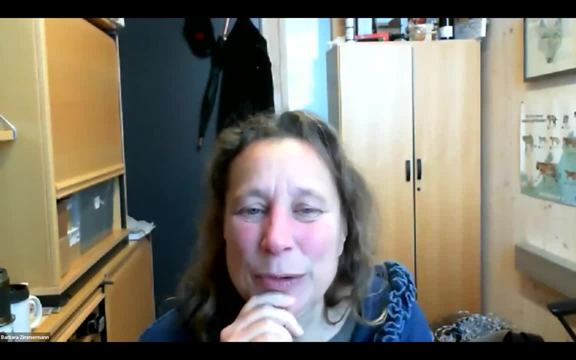 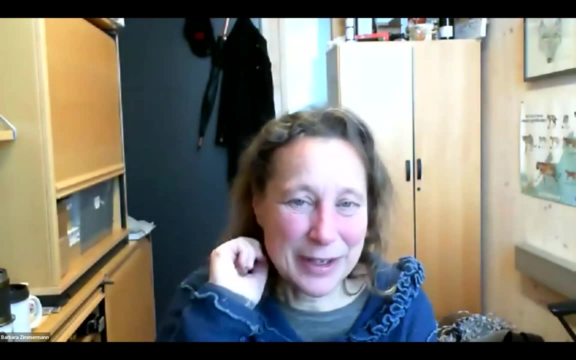 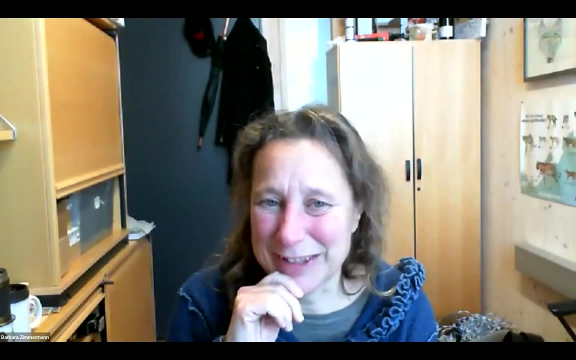 and another colleague of mine uh supervising them, uh looking into the beaver moose uh relationship. so in the same study area where we have done all these uh studies on the moose densities and what i've been presenting, if now also this year, we've had students out- 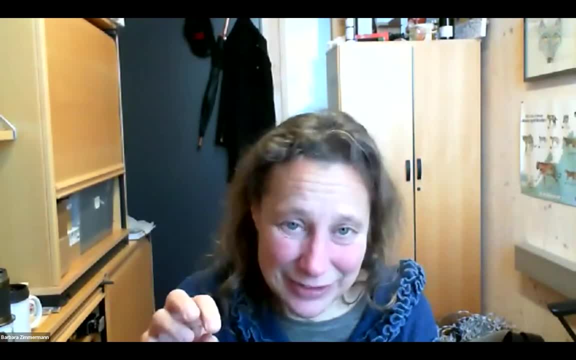 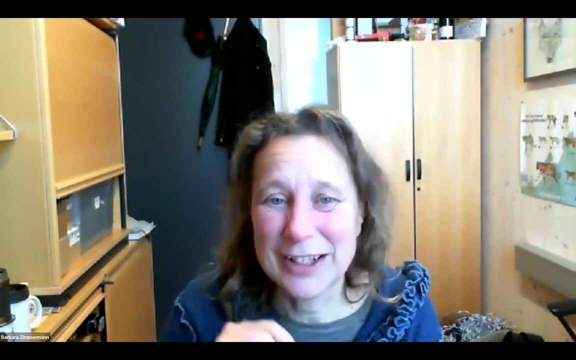 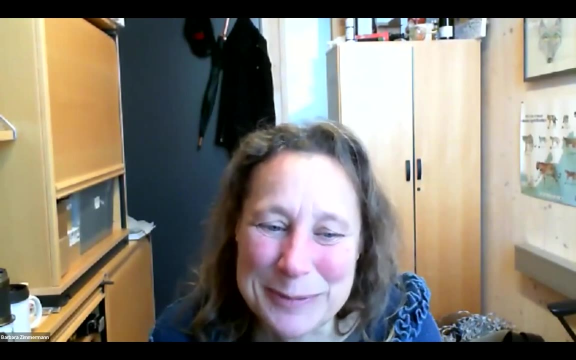 uh registering uh beaver activity, and we are also then looking into how this radio GPS column moves are using waterways. so it will be interesting, but i can unfortunately not answer the question yet, so hopefully we will have an answer in a few years from now. thank you. 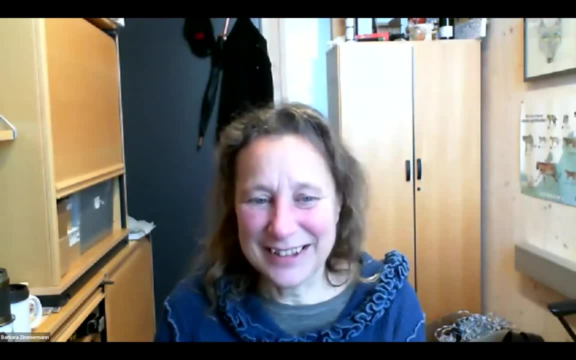 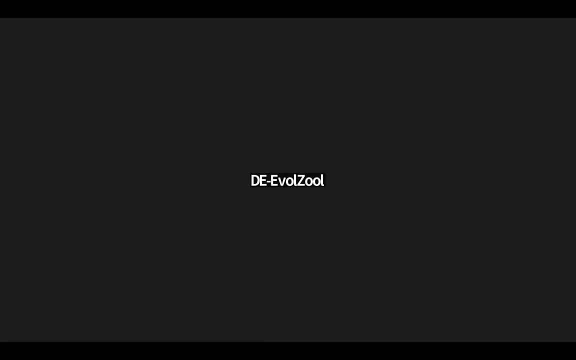 okay, then, i think we are done. yeah, i think we are done. okay, okay, thank you everyone. have a nice day, bye, bye, bye, bye, bye.